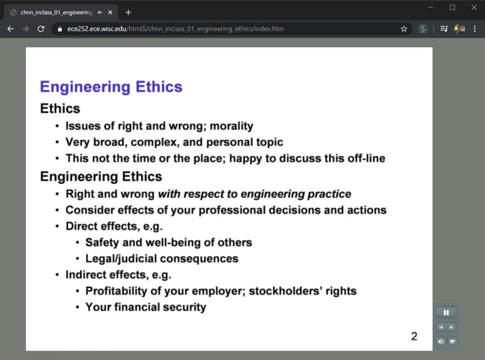 is a very important area that traditionally has not really been treated very well, or perhaps even at all, in engineering curricula, And so we try to do a little bit more of that these days, and we have for that reason a brief report. 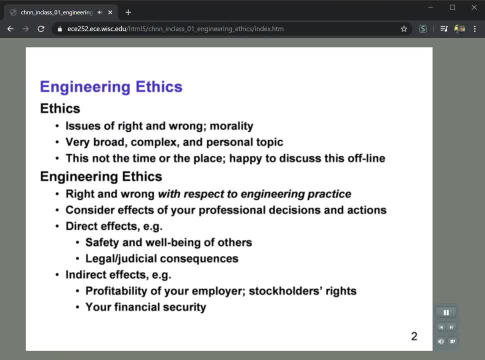 I'm going to give you a little bit more detail on that in just a few minutes, and then I'll get back to you with a little bit more detail on what we're going to talk about in the next couple of weeks. So I'm going to give you a little bit more detail on what we're going to talk about in. 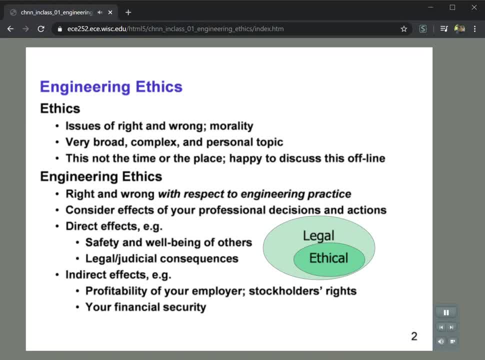 this one-week unit on this topic. in this course, You should be aware that what's considered ethical and what's considered legal are not necessarily exactly the same thing. It's clear that in many cases, the set of actions that we would consider to be ethical are a 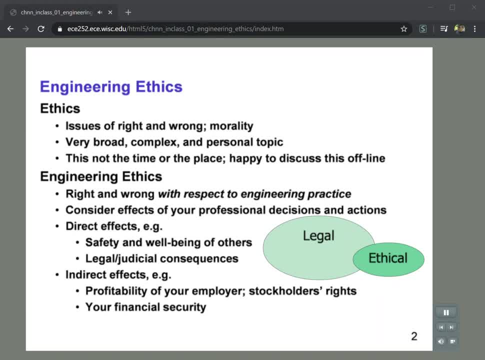 strict subset of the things that we would consider to be legal, But that's actually not sometimes the case. Sometimes there are things that we would consider to be ethical, based on our own personal standards, that might actually be legal, But that's actually not sometimes the case. Sometimes there are things that we would consider to be ethical, based on our own personal standards, that might actually fall outside the realm of legal activities. 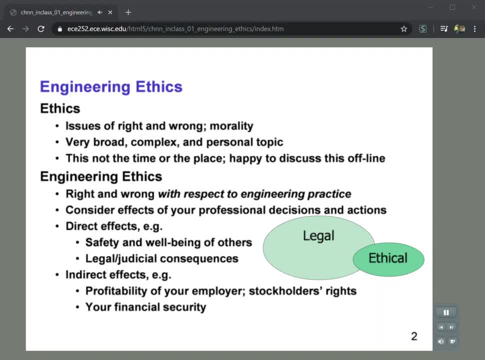 It is especially in this domain, when we're dealing with things that perhaps fall into the space of actions that we might undertake, that we would consider to be ethical but the legal system probably would consider to be illegal. We have to be very, very careful in making sure that we do things and consider the consequences of our actions before we pursue them. 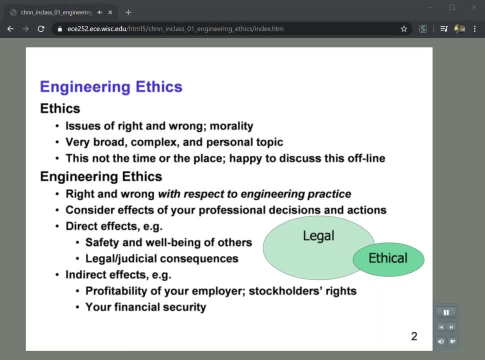 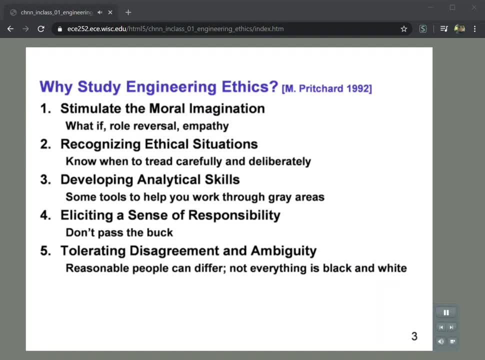 So we'll talk about a few ways to do that, A few ways to a few tools that we can use to help us make better decisions. within this context, One of the things we can really think about is: you know, why is this even important? 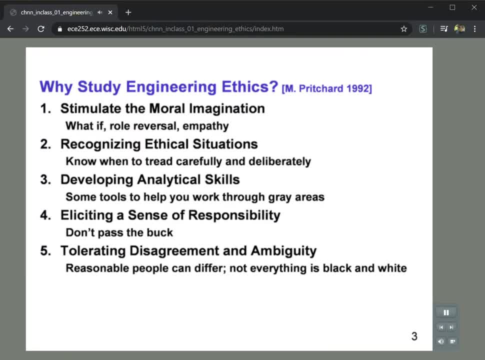 You know who cares. We're engineers, We design things, We build things. Are there really any ethics, ethical issues at play? The short answer to that is yes, there are. You will inevitably encounter scenarios and situations in your professional career as an engineer or as a computer scientist that will require you to consider. 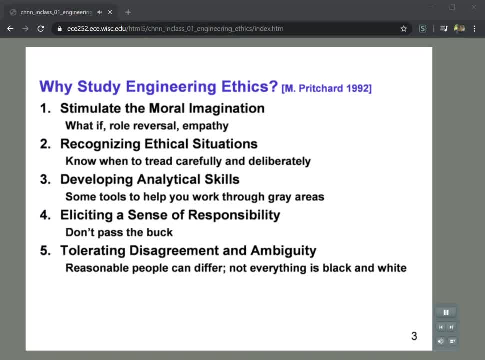 Some of the issues that we'll be talking about in this lecture. So here's a list of five reasons why you may want to think about studying engineering ethics and spending a little bit of time dwelling on this issue and perhaps being a little bit introspective and trying to think a little bit about what it is that makes you make the decisions that you personally make. 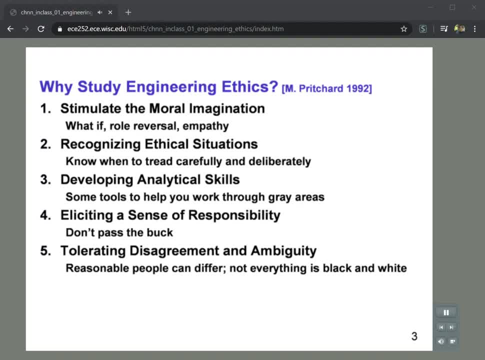 What are the ethical principles and so on that you apply in your own life? So the first reason here, First reason to study engineering ethics, would be to stimulate the moral imagination. So if you've never done this, it's useful to be able to do this, to basically do some role playing, to create what if kinds of scenarios in your head that says: what if it was me in that situation? 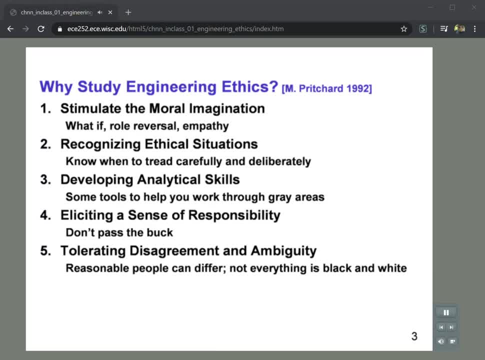 What if I was actually on the receiving end of this action that I'm about to perform that may or may not have ethical implications and repercussions? and to develop sort of a sense of empathy for the situations that others might find themselves in. Second reason would be to help you recognize ethical situations so that you'll recognize and be aware that you've now entered into the realm of decision making, where ethics come into play. 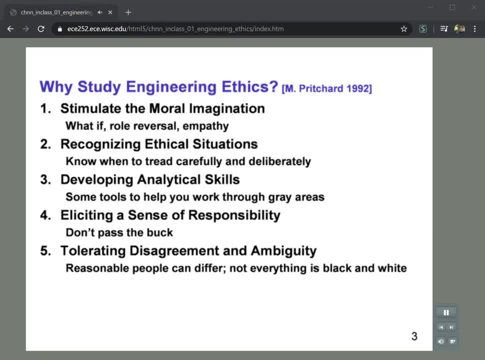 And you should probably be quite deliberate and careful about the path that you choose to follow, Whereas most of the time- truthfully, probably the vast majority of the time- in our engineering work, we don't have to grapple with difficult ethical situations. 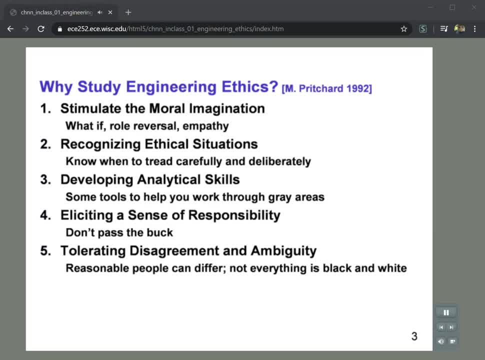 The third reason to do- to spend a little bit of time studying engineering ethics- would be to develop some analytical skills, And we'll talk about a few of those tools that will help you work through some of the gray areas. Fourth reason would be to elicit a sense of responsibility. 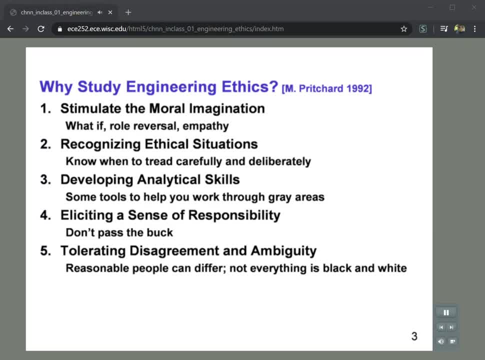 Oftentimes the easiest response to an ethical quandary is to pass the buck, is to say: well, that's not my problem. My manager or my manager's manager, or the CEO of my company or whoever has already made the decision To do this or to not do this. 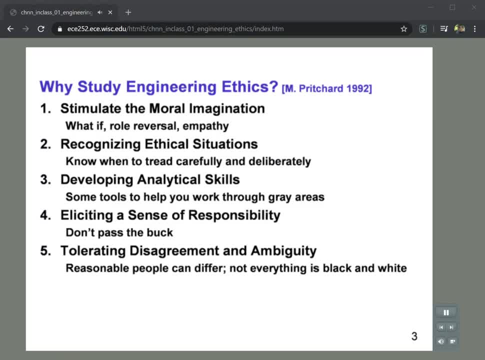 And I'm just going to do what I'm told and be a good foot soldier, And that's not always the right response. even if, ultimately, the action that you decide to pursue falls in line with that reasoning, It's still the right thing to do: to have a personal sense of responsibility with regard to personal actions as well as corporate actions by your employer. 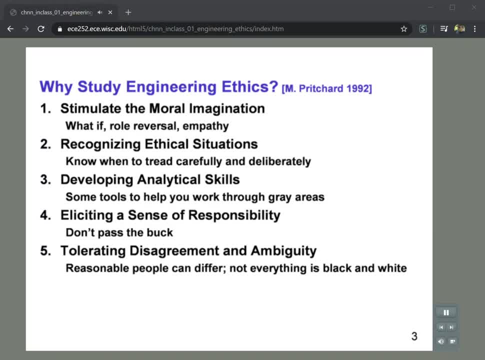 So that, so that you are, You're not just being a good foot soldier, but you are standing up for the things that you need to stand up for when they become important enough to stand up for them. So that's a that's a good reason- is to just develop an awareness and a sense of responsibility for some of these issues as they come into play. 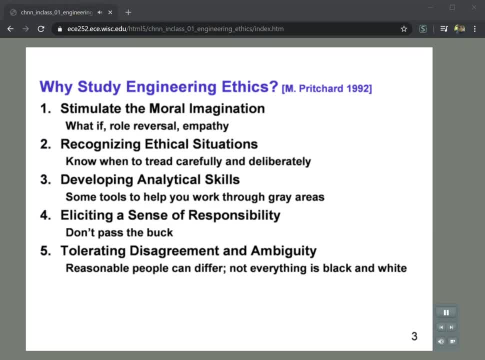 And finally, just studying this issue and understanding that there are many different perspectives that people can have will help you develop a tolerance for disagreement and ambiguity. Not everything is black and white. There are topics and areas in which reasonable people can differ, And spending a little bit of time thinking about this and understanding this whole problem will make you feel more comfortable with that idea. 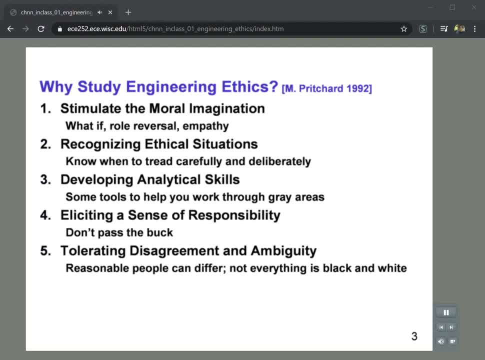 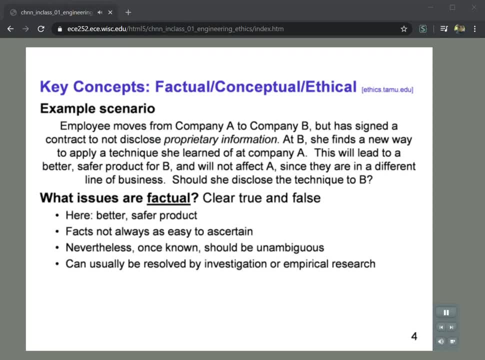 Sometimes people just don't feel comfortable with the idea that that the opposing viewpoint on a particular topic can actually be reasonable. One of the key concepts in the understanding of ethical situations is to try to differentiate between What, in that scenario, is a fact, What is factual. 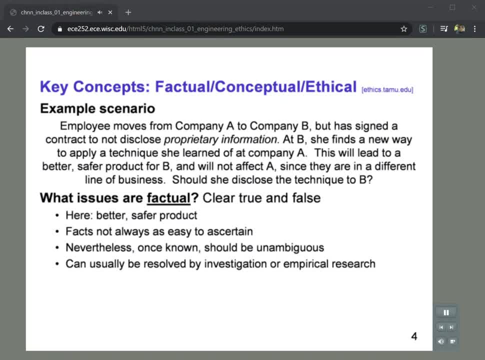 What, in that scenario, is conceptual And so largely a matter of definition and agreement, And what is in what is, in turn, ethical. So we want to try to identify Aspects of the scenario that we're considering or the situation that we're faced with that fall into these three categories, so that we can isolate the ones that really are just a matter of our ethics. 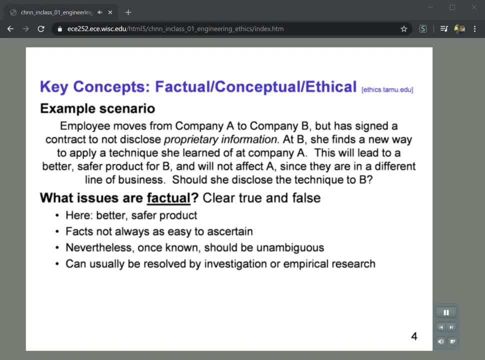 And we can focus on Those rather than on the factual and conceptual issues. So we'll do that. Do this analysis in the context of an example scenario. So let's say, an employee moves from a company- one company A- to another company B. 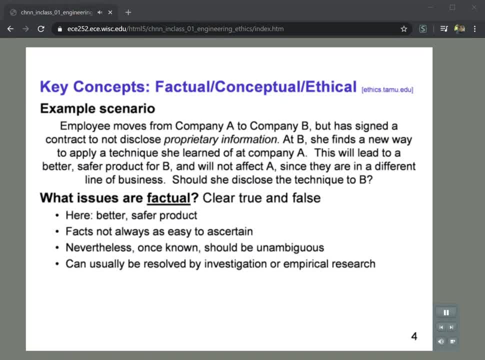 But as part of their employment with the first company, they've agreed not to disclose any proprietary information. This is a pretty standard thing that companies will make you do. Anything that you learn while on the job there has to stay there. You can't take it with you to the next job. 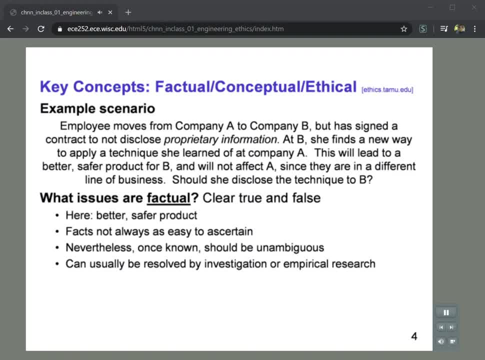 And apply it there. However, this employee, in this situation, finds a new way to apply the technique that she learned at company A at company B. This will help company B build better, safer products And it really will have no effect on A because they're not really competing with each other. 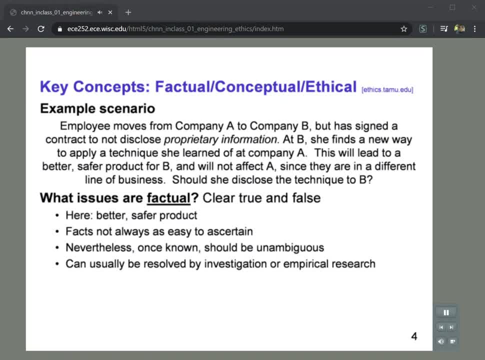 She's moved from one industry to a different industry and a different line of business, And so there really is no- There really is no issue of giving company B An unfair advantage against company A, Since the two companies don't actually compete with each other. 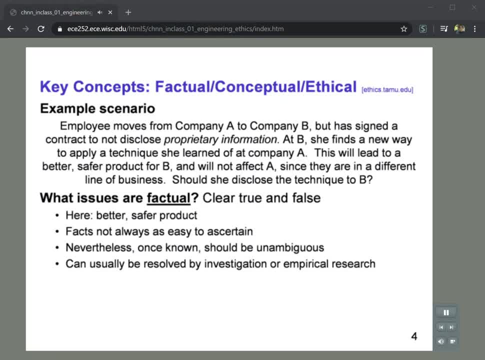 So the question is, the ethical quandary is: should she disclose the technique to B? So there's many issues at play here. We'll focus first of all on the factual issues. So what are the issues in this scenario that are factual? By factual we mean they're facts. 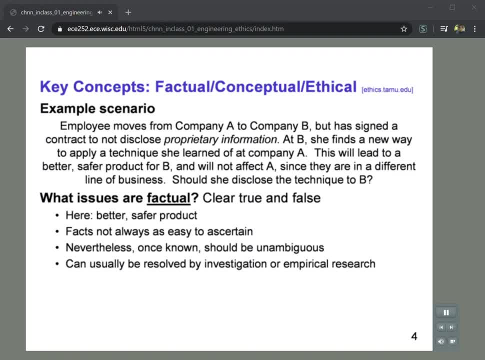 They're clearly true or false. The only real fact here is that applying this technique will lead to a better success. It will lead to a better, safer product. There's no question about that. There's no doubt about that. However, just because it was easy in this case to figure out what the facts were, 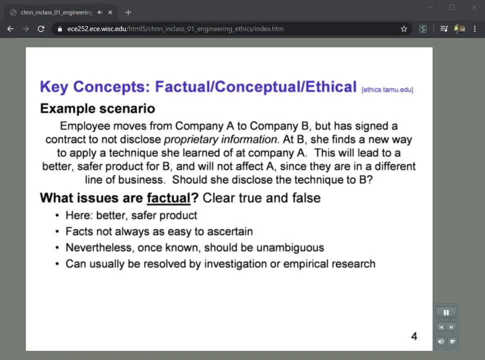 That's not always going to be the case. Depending on the scenario, facts can be difficult to ascertain. They might be historical facts, There might be different people involved who might have different recollections of what happened, So there might be some uncertainty there. 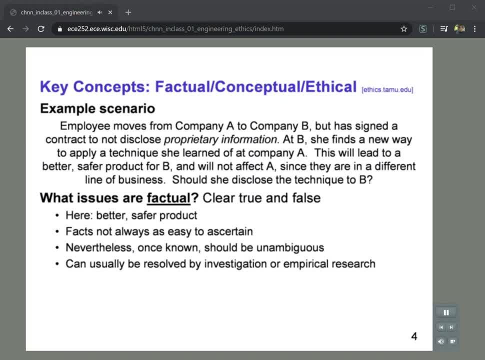 But in general it's the case that these factual issues should be things that we can extract out Fairly unambiguously And we can usually resolve them by further investigation or by doing some empirical research to validate or verify any assertions in the scenario. 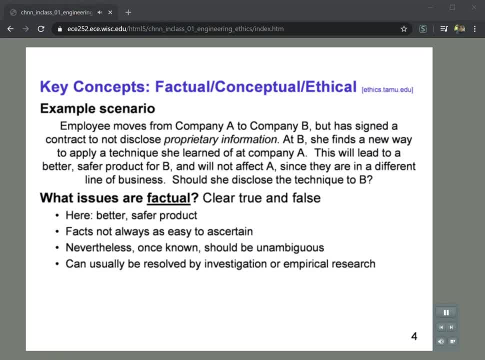 So these are the things that we, as engineers and as mathematicians and as scientists, should be pretty comfortable with, trying to get to the bottom of the factual issues in a scenario like this. The next category is really the conceptual issues. So, again, conceptual issues are really you can think of them as they're a matter of definition. 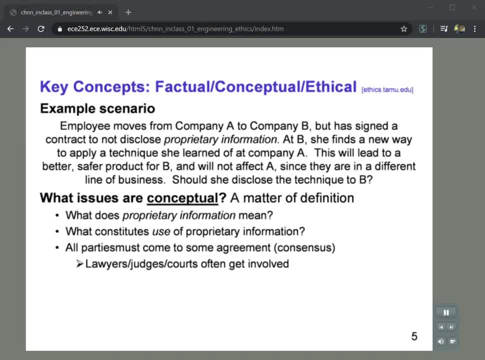 So in this particular instance, we have the phrase proprietary information, Which appears in the employment contract that this employee had signed at the first employer, Company A. So the question really becomes then: what does proprietary information mean If the information that she acquired while she was at Company A is something that she perhaps could have picked up? 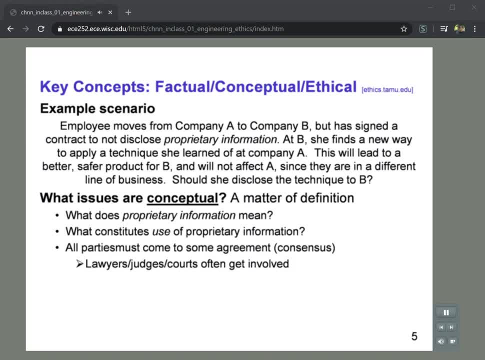 By taking another course somewhere, Or perhaps could have picked up by doing some literature search. Is it truly proprietary? Probably not. So proprietary would have to mean something that's normally called a trade secret for the company that really isn't known anywhere else. 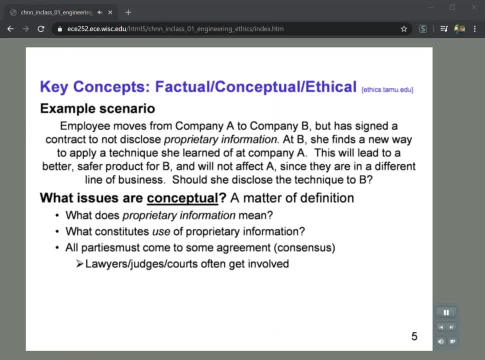 And could not be discovered anywhere else. So there has to be some kind of definition of what it is that we mean by this proprietary information. Furthermore, we have to have some understanding of what the use of proprietary information is, What it really means. 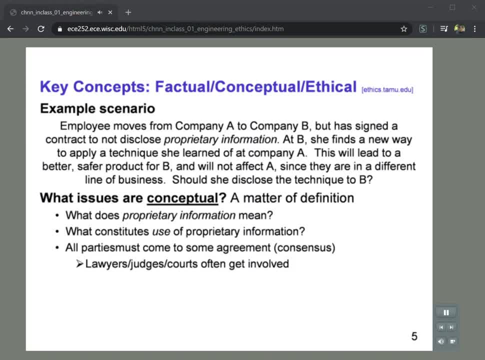 What constitutes use of proprietary information. I think in this case it's pretty clear. applying that information to the development of a different product, Development of a different company, Would probably be a reasonable definition of use of proprietary information. In general, these conceptual issues have to be unearthed or have to be agreed upon by everyone involved. 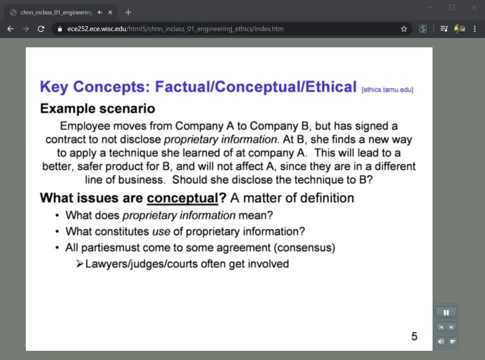 So there has to be some kind of consensus. Whether it's a true consensus, Whether it's one that's imposed through a trial process by a judge or a jury, It's kind of dependent on the scenario, But it is unfortunately the case that quite often lawyers and judges in courts will get involved to help establish these conceptual issues in these scenarios. 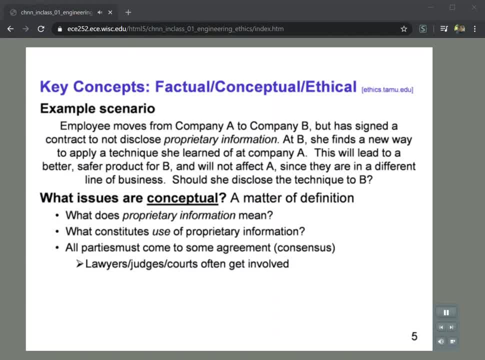 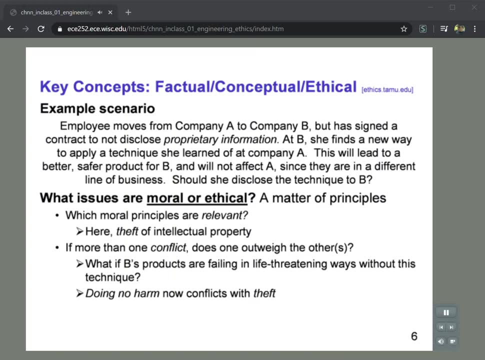 If they actually escalate to the point where the two companies in question will go to court Over the events that have transpired. The final category, then, is pretty much what's left over. So these are the ethical issues. So what are the issues at play in this scenario that are ethical or moral? 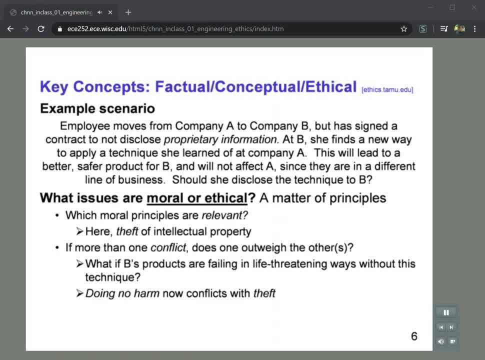 Well, anything that's moral or ethical is really a matter of principles. So, given some set of ethical principles that a particular individual desires to adhere to, The question really then becomes which of these moral principles are relevant to the case at hand. So in this particular case, the moral principle is really theft. 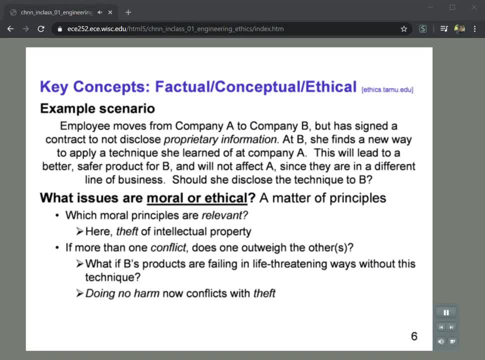 So is it okay to effectively steal intellectual property from one company and hand it over to another company? It's pretty straightforward in this case, But again, quite often there's more than one moral or ethical principle that comes into play. For example, we could expand on the scenario and say what if it's the case that the product that B manufactures? 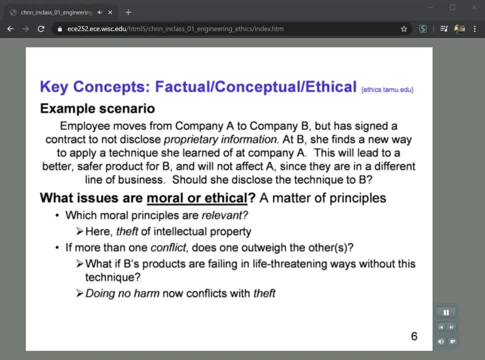 Is actually failing in a life threatening way without this technique. So actually, the end users- perhaps it's a medical device? The patients are actually at risk of life because of this deficiency in the product, And now this employee really knows how to improve the product. 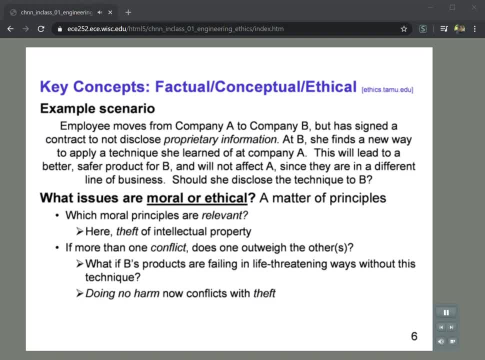 As a result of this proprietary information, she picked up at another company. How does that change this scenario? And it does change it dramatically. The ethical principle comes into play. Many of us would like to think that there's an ethical principle that could be summarized as doing no harm. 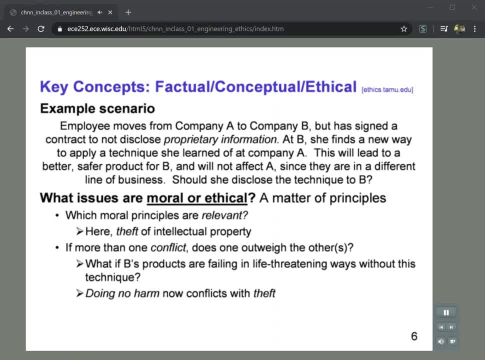 We should do whatever we can to create products and so on that will not harm their users, To the extent that that's possible. So we have a doing no harm ethical principle and we have a theft principle, And the two of them now conflict. 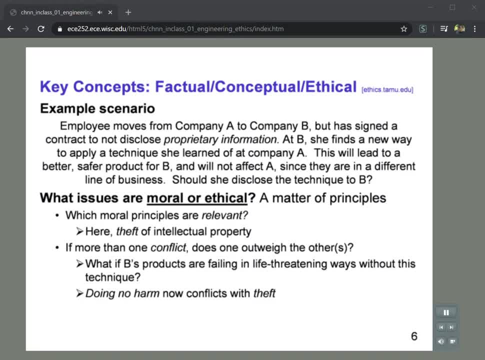 And in order to resolve this question, We would now have to somehow weigh these two principles Against each other, Weigh the relative effects of violating one of them Against the benefits With respect to the other one, And we'd somehow have to juggle these priorities now. 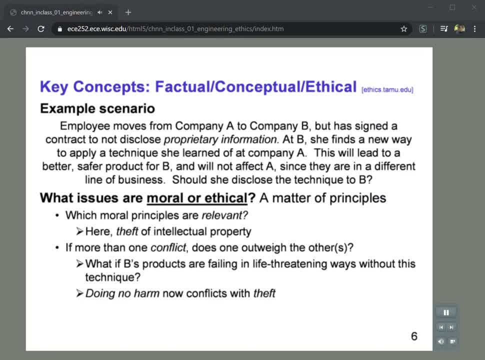 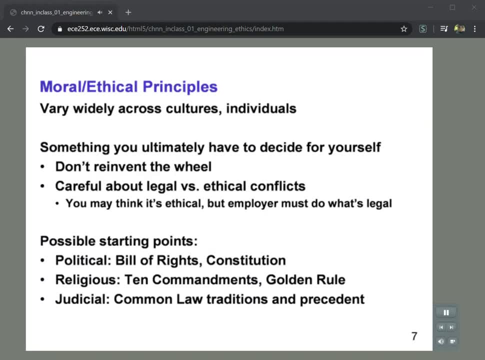 These ethical priorities And reach a conclusion, So we'll talk a little bit about some ways to help us work our way through that reasoning process. Before we do that, though, Let's talk a little bit about what moral and ethical principles are in general. 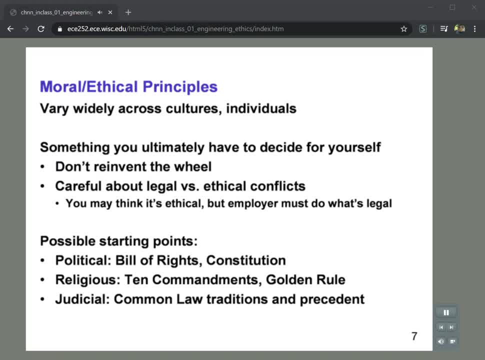 Obviously, these are something that are going to be To vary widely across individuals And across cultures, And ultimately they're something you have to decide for yourself. It's part of the process of growing up and becoming an adult Is to basically look around and examine the ethical and moral principles that you've been exposed to. 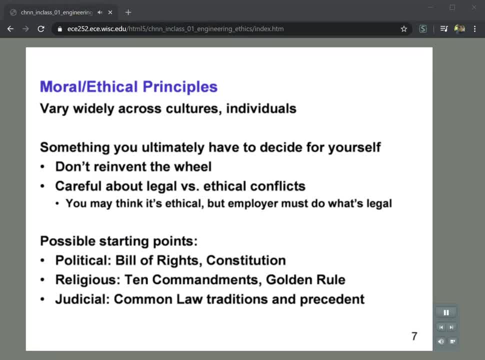 Through your childhood And decide which ones are the ones that you're going to choose to apply to your own life Or to try to follow in your own life. Now, the only advice I can give you here is: don't try to reinvent the wheel. 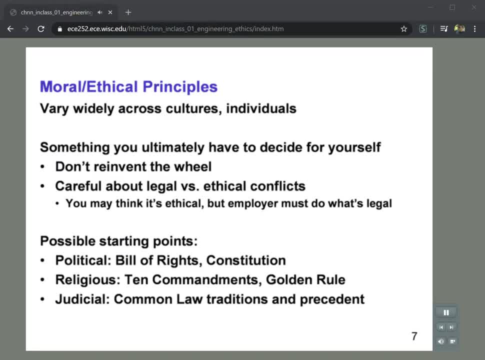 Humans have been living in organized, structured societies for thousands of years, And the moral and ethical principles that have been well established in those organized societies Are there for a reason, And it's generally not a good idea to throw everything out and start over. 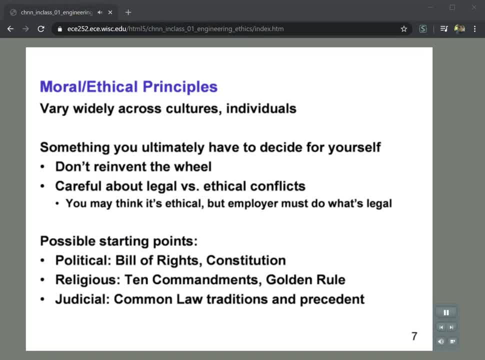 But a much better idea to just carefully examine the set of principles That you see, perhaps your parents or your relatives living by, And your peers, And then decide whether those are the ones that you also want to adopt. One area in which we understand: 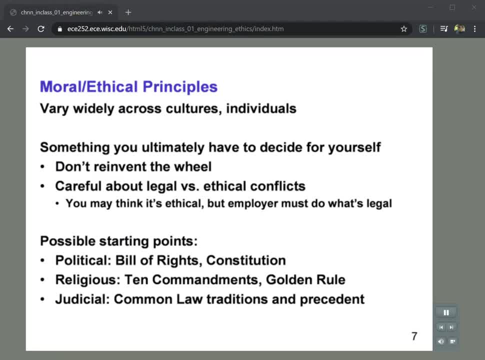 To be particularly careful here, though, is Any principles where there are conflicts between what you might view as ethical Versus what might actually be legal in the country that you're living in. So there may be actions and things that you may think are ethical. 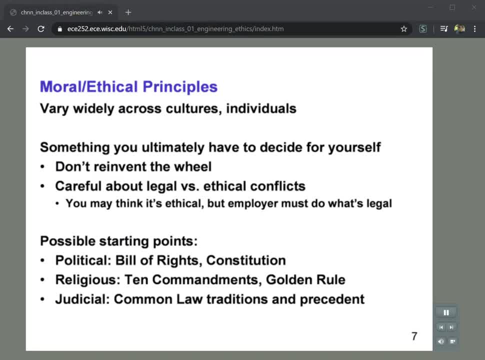 But your employer is going to be constrained to doing what's legal, And so you have to be very careful about engaging in any activity That you might consider as ethical, Again in your professional capacity, But that your employer Would possibly disagree with. 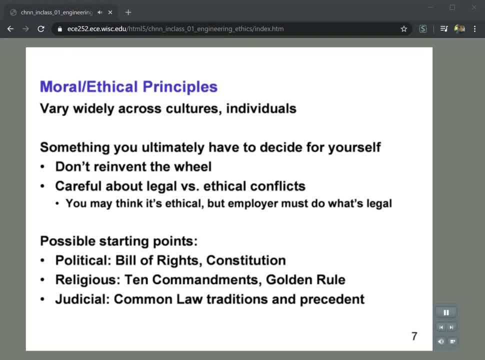 Because of the law of the land, And you have to realize that there will be repercussions for that. Your employer is not going to respond positively To you doing things that are illegal, Independent of what your ethical view of those actions may or may not be. 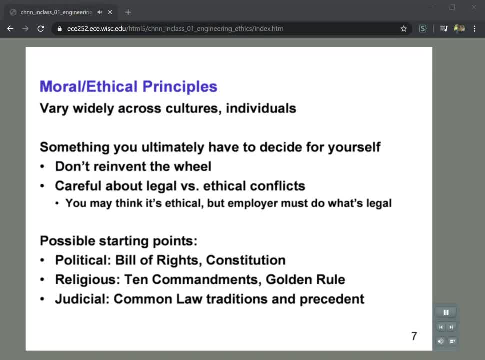 So, Okay, What are some possible starting points for building up a set of moral or ethical principles That you might choose to apply in your professional life, While you can start in the political realm, Maybe with the Bill of Rights And the US Constitution? 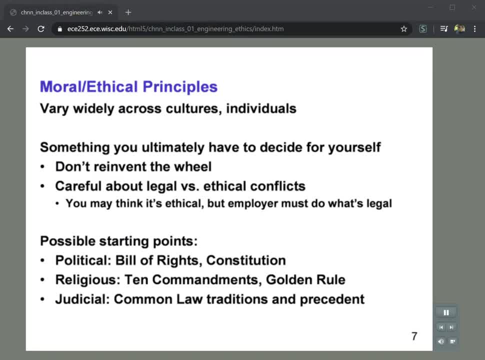 You could start in the religious realm, Maybe the Ten Commandments Or even something simpler, The Golden Rule. Or maybe in the judicial realm You can look at something like English Common Law, Which dates back hundreds of years And has established many traditions and legal precedents. 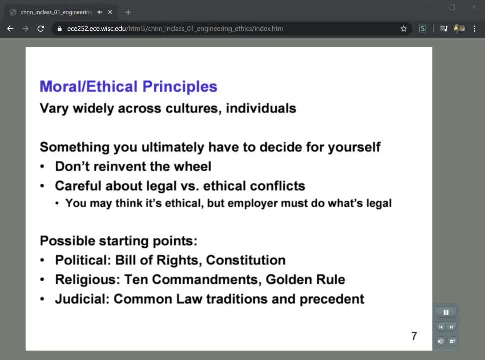 Governing the interactions And the rights and the responsibilities of citizens. Again, This is a very broad topic, A broad topical area, And we're not really going to dig too much deeper into what particular moral or ethical principles You might choose to have. 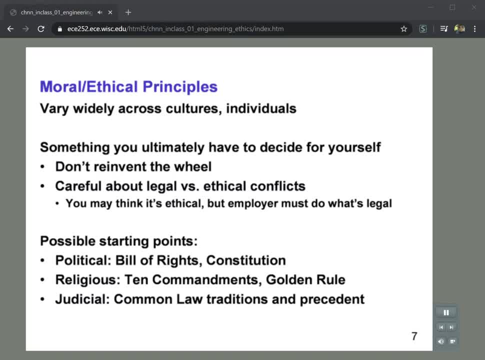 Rather, we're going to stick more on the analytical side And present you with some tools and some examples To help you along in the process of thinking about this, Rather than trying to lead you to any particular correct answer In this domain. Okay, 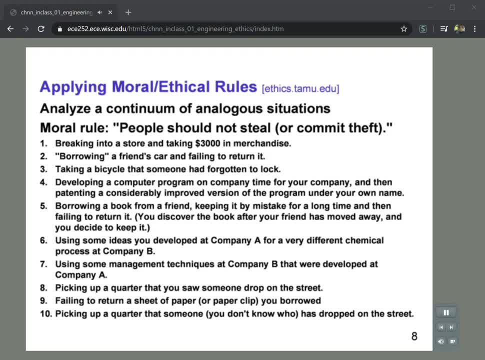 Going back to the context of our earlier discussion, For example, Once you have identified a moral or ethical rule or principle that you feel is relevant That is potentially being violated in the particular scenario that you're trying to resolve, It can be useful to try to create a continuum of analogous situations. 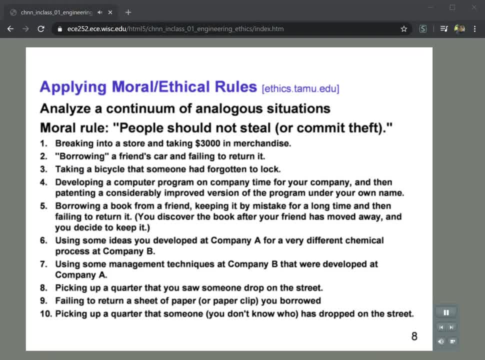 So try to create a set of situations that range from clear and obvious violations of that principle At one end- So these would be the first few on the list here- Versus ones that are progressively more ambiguous, Until you finally get to cases where 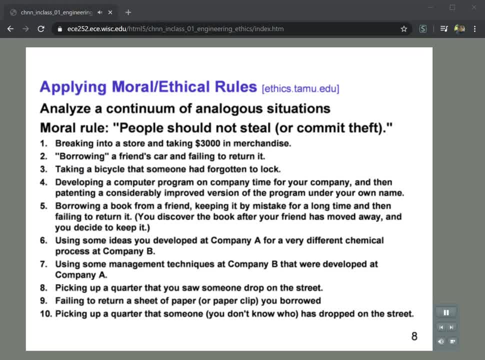 Yeah, You might see that somebody would view this as being a violation of this ethical principle, But definitely most people would probably say: Who cares? That's no big deal. So just picking a few from this list, Which I encourage you to read in more detail: 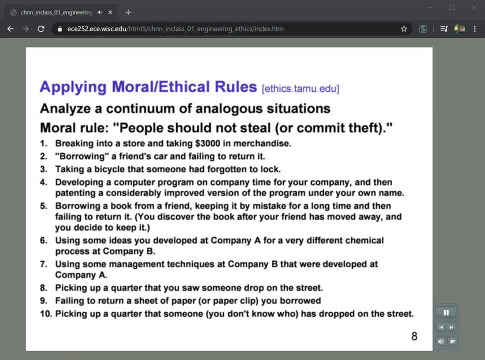 Obviously at the top of the list. If I break into a store and I steal $3,000 in merchandise, I don't think there are too many people that would disagree with the statement Or would disagree with the fact that this is a violation of a moral principle. 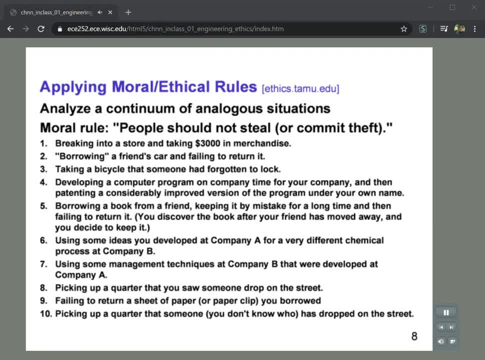 That says we should not steal or commit theft. The second one here: Borrowing somebody's car and failing to return it, That's also pretty obviously in violation of that ethical principle. But if we go further down And get to kind of the other end, 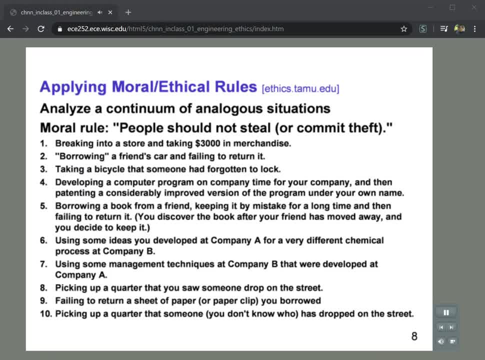 Number 10 here If you pick up a quarter that you find on the street, Well that's probably You wouldn't find too many people that would try to say that that's actually stealing. And as you go up to 9 here, 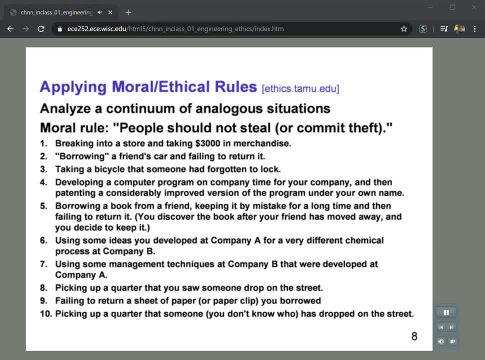 Failing to return a sheet of paper, A paper clip you borrowed. Okay, that's such an inexpensive item That it really sort of falls into a gray area: Number 8.. If you pick up a quarter, But you actually saw the person drop it. 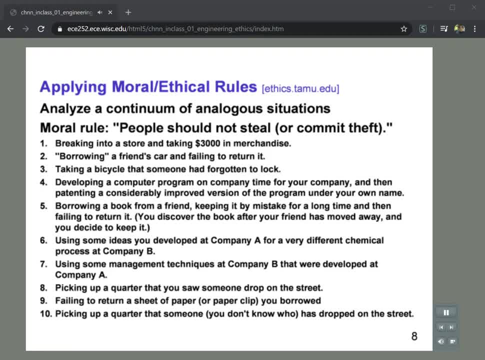 Well, now it gets a little iffy. Should you actually chase that person down And return their quarter to them, Whereas a quarter is such a small amount of money That again, It's really sort of nonsense To do that. So you create this kind of continuum. 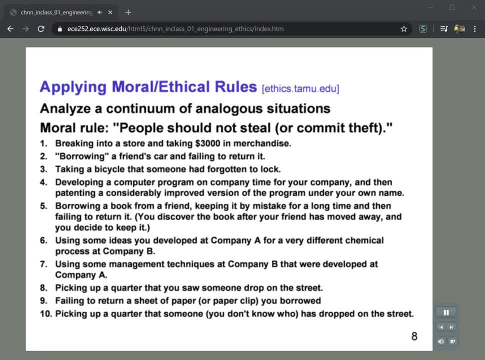 Of analogous situations, And then you actually try to place The situation that you're facing Into this continuum And that gives you a sense Of how black and white, How clear is it, How clear is the situation Versus? how much ambiguity is there? 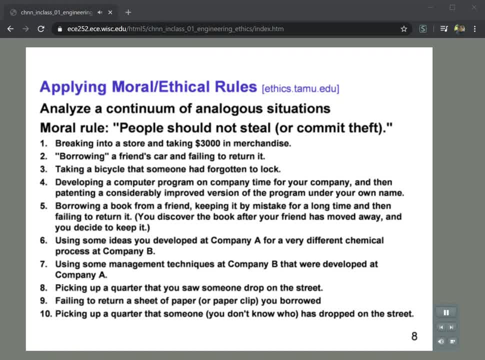 And how much sort of? How much are you into the gray areas of this ethical principle? So in this particular example We put the example that we were talking about Using some ideas you developed at company A For a very different process At company B. 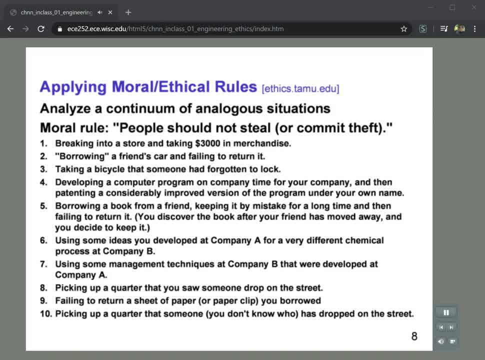 In the middle here At about number 6.. So this is sort of you know, Closer perhaps to the end of End of the continuum, Where most people would think it's probably okay, And a little bit further from the end. 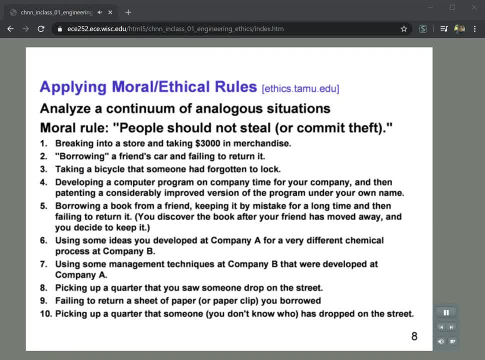 Where most people would unambiguously declare That it's a violation of this ethical principle Against stealing. So again, This is really not an algorithm That will give you an absolute, definitive answer As to whether what you're doing Is a violation of that ethical principle. 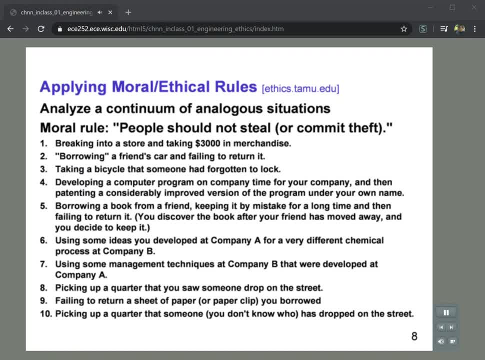 Rather, it's a way to help you Think about it in a little bit more depth And to generate some sort of introspective thoughts That will perhaps lead you To a more well-informed And more likely So a decision that will. 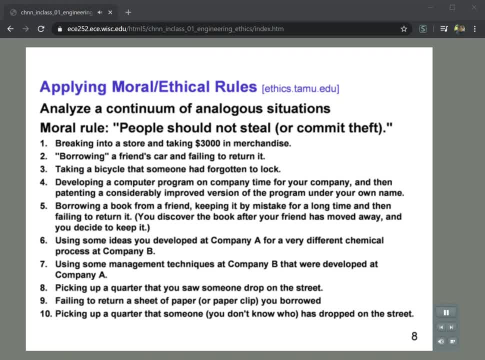 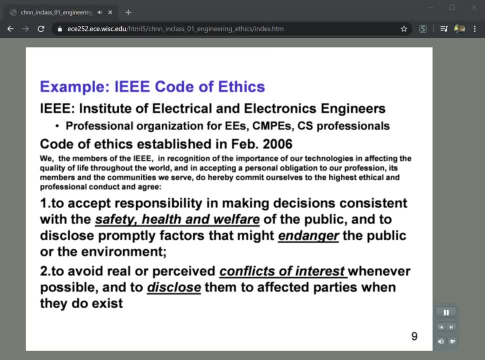 You'll more likely be comfortable with In the long run. One example that can be helpful here Is to go through an actual code of ethics That's been created by the IEEE, Or the Institute of Electrical and Electronics Engineers. IEEE is an organization that I belong to. 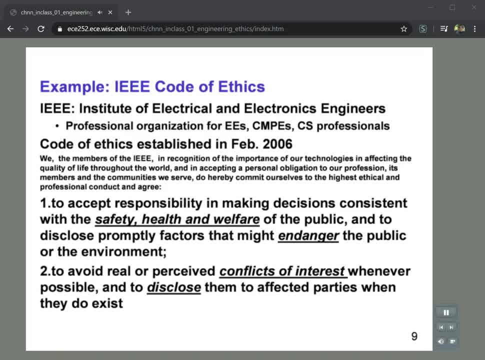 It's the professional organization For EE's Computer engineers And computer science professionals, And just a few years ago, In February 2006.. They actually assembled a committee And sat down And decided to create a code of ethics For our profession. 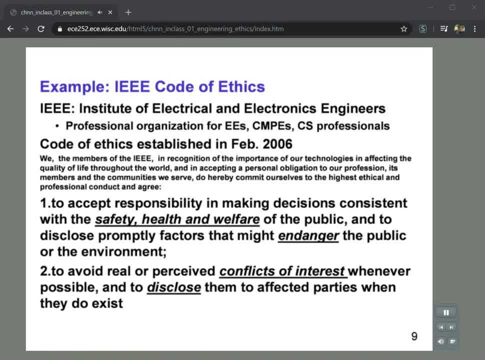 Now, this code of ethics In and of itself Is not something that's, in my view, Particularly good. It's kind of a jumble of concepts And philosophies And suggestions And so on. It's not. It's perhaps not the greatest example. 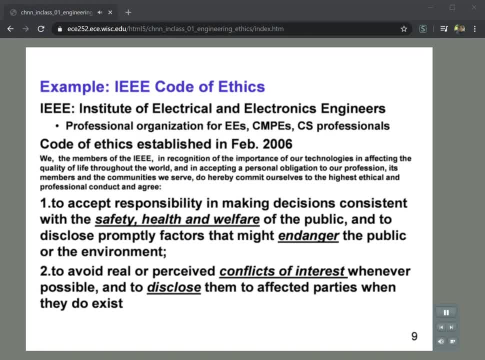 But it does touch on a bunch of areas That are relevant and important, So it's worth going through. So let's go through this. So the first one says To accept responsibility In making decisions consistent with the safety, Health and welfare of the public. 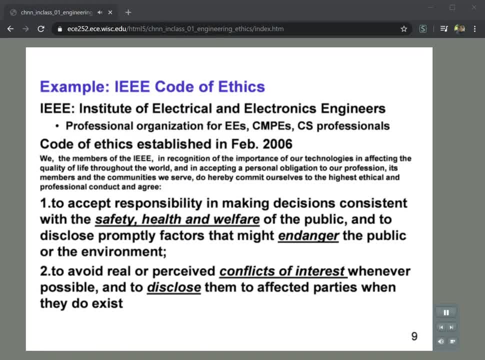 And to disclose promptly factors That might endanger the public Or the environment. So this is specifically having to do with Engineers who are designing products That could have an impact on safety, Health and welfare And could potentially endanger the public, And the code of ethics just calls for behavior. 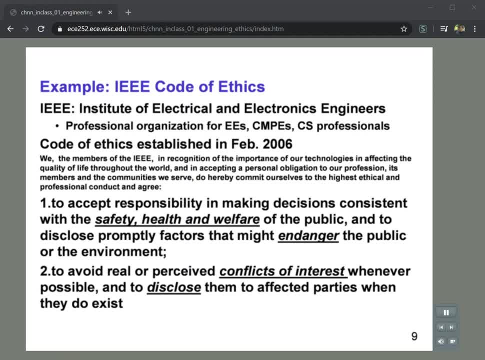 That will minimize these safety impacts And will disclose factors That might lead to dangerous situations. Fairly straightforward, obvious stuff. The second one here is To avoid real or perceived conflict of interest Wherever possible And to disclose them. So conflicts of interest are. 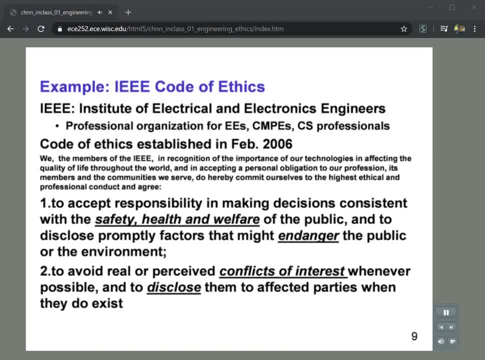 Usually the kind of situation is where, Let's say, you are responsible For making a purchasing decision With respect to components That you're going to use For a particular engineered design That you're working on And you decide to purchase components. 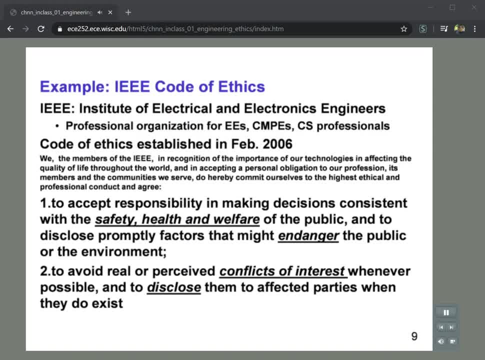 From a company that you have an ownership interest in, Or perhaps is owned by a family member. So you're basically going to steer Your company's business To another company That you also have a financial interest in. That's an example of a conflict of interest. 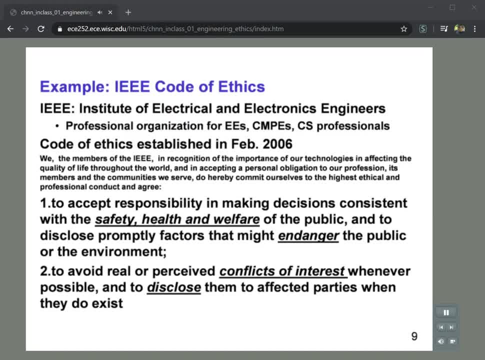 So these are something that Come up quite often And are something that You have to deal with honestly. So, again, avoid, real Avoid them if possible And if they do exist. And you really can't avoid them Because, let's say, 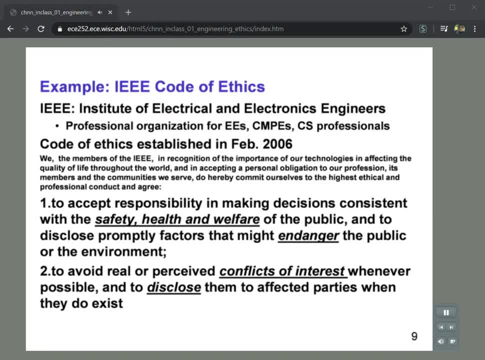 Truly, the best product That you can use In your own engineered design Comes from an entity or company That you have a conflict of interest with. Well, if that's the case, Then just make sure to disclose that And put it out in the open. 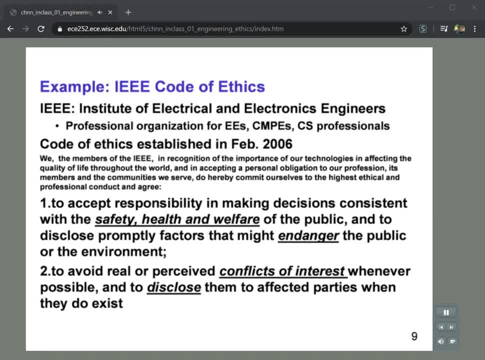 So that this isn't something That will be discovered later And you'll be accused of doing something dishonest Much later. it's much better. The right thing to do is to make sure That this is all publicly disclosed up front To all the affected parties. 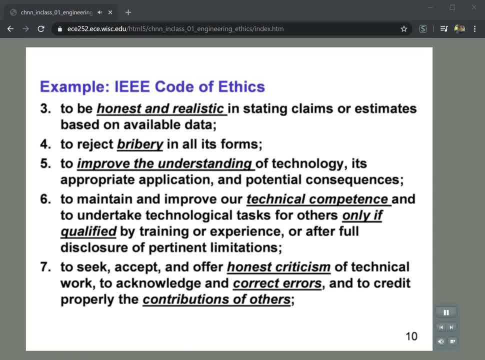 So that's the first step. The third clause of the IEEE code of ethics Then calls us to be honest and realistic In stating claims or estimates Based on available data. So one of the big jobs That we, as engineers, will do. 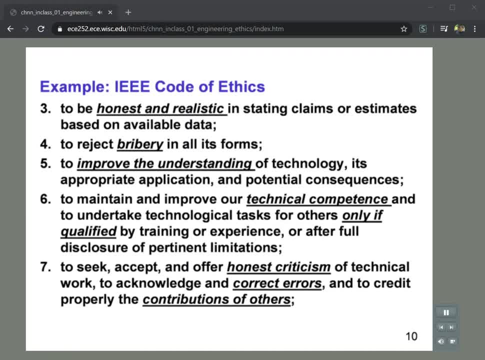 Is. we will be asked to estimate Or make claims about Particular attributes Or features of products, And there's often a temptation To oversell things, To basically claim That this new processor Is going to be the greatest thing. 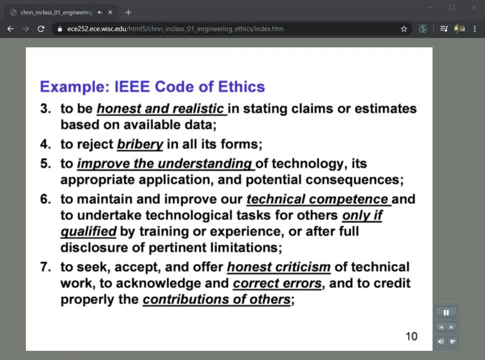 Since life's spread, It's going to be twice as fast, Or use one tenth the power, Or whatever the metric might be, Relative to its competition, And so the IEEE code of ethics Simply calls for us, as engineers, To always be honest and realistic. 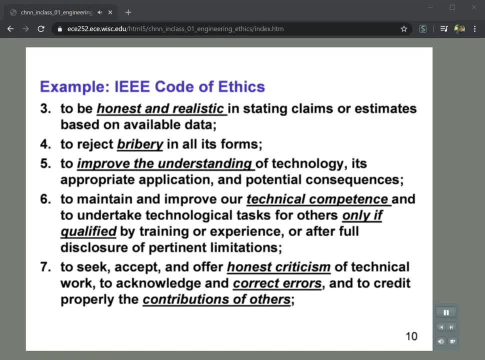 In making any claims or estimates. The fourth one is also fairly straightforward. We should reject bribery in all its forms. So if someone offers you Compensation in order to influence a decision, Again this is similar To the conflict of interest situation, But this is an explicit case. 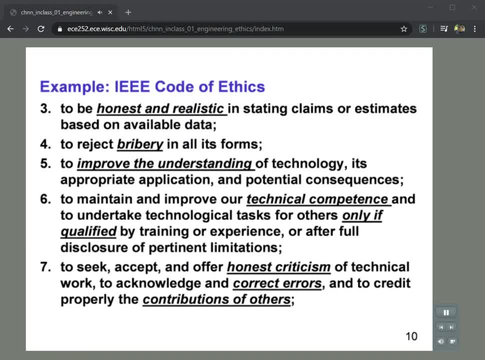 Where someone is actually offering you money To steer your decision in a particular direction. That's something that we should always reject. Fifth, We should seek to improve The understanding of technology And its appropriate application And potential consequences. So this is sort of a civic clause here. 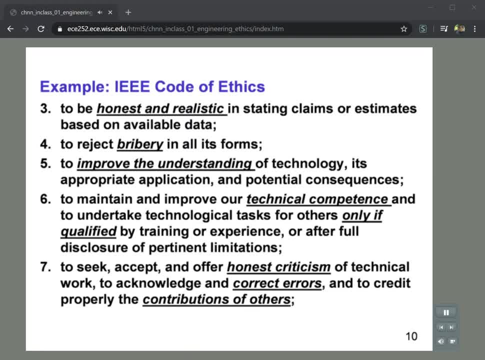 That says it's part of our civic responsibility To help others in society Who may not have the technical background Or the understanding of a particular technology That we have. We're responsible, We're on the hook To help people understand. 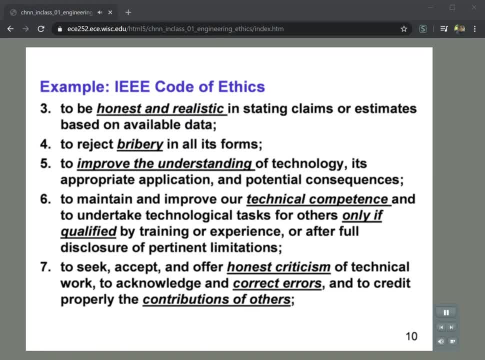 We should be willing to stand up In the marketplace of ideas And educate people And help them understand That a particular technology, What its advantages and disadvantages Might be, in an honest fashion, So that decisions that others make, Especially decisions that politicians might make, 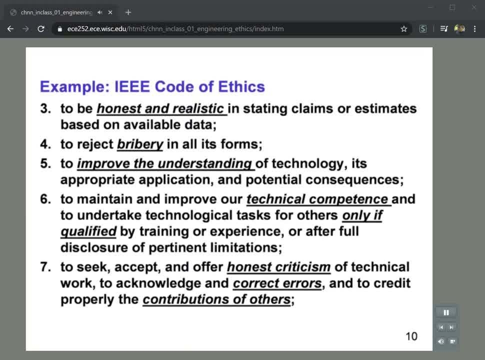 Would be well informed decisions Rather than poorly informed ones. The sixth clause then Calls us to maintain and improve our technical competence, And to undertake technological tasks Only if we're qualified By training or experience, Or again After full disclosure of any limitations. 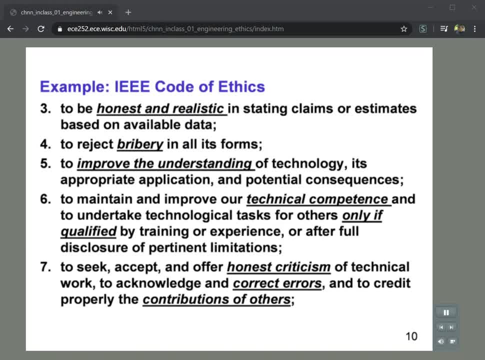 So this really has to do with the fact That sometimes we'll be asked to work on things Or design things That we really aren't qualified To work on or design. So first of all, We should make sure we maintain our technical competence. 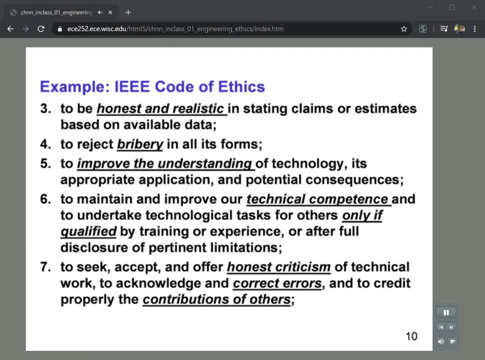 So that, as things change in our industry, We don't just cling to the things that we learned, You know, 20 years ago, When we were undergraduates, But we continually educate ourselves So that we remain competent and up to date. And then again, 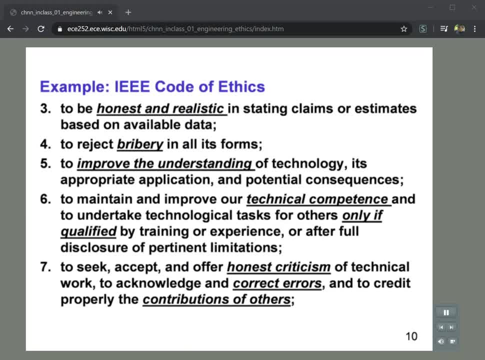 When we're asked to work on a particular project, We have to make sure that We actually have the skills in the background To undertake that task, When we are actually qualified for it Or if Whoever is insisting that we do this. 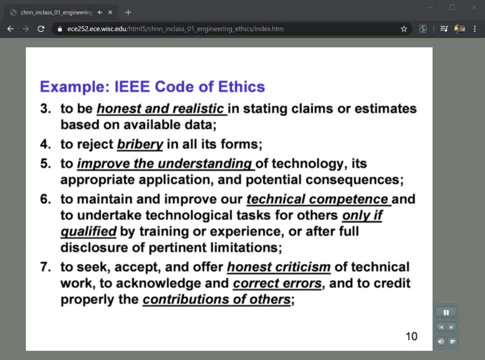 Continues to insist, We at least fully disclose our limitations To the project. The seventh clause here, then, Is really about Providing honest feedback Or honest criticism, Both to accept it And to offer it to others, So that, when we're asked to review the work of others, 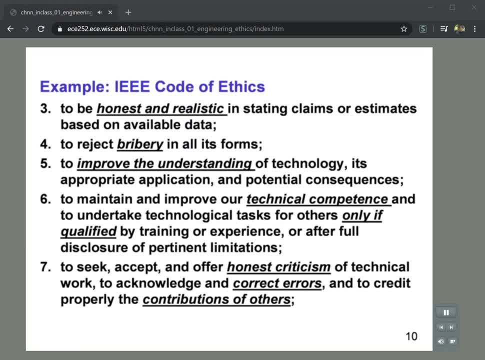 Or when others are reviewing our work. We will honestly acknowledge any errors And correct any errors, And we will also credit properly The contributions of others. So if there were six of us That worked on a particular project, We would often claim all the credit. 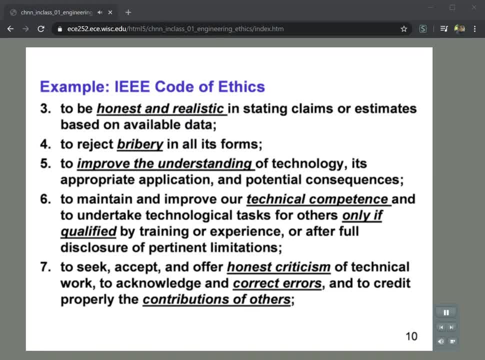 I should fairly allocate credit And acknowledge others contributions. This is again something that The code of ethics calls us to, But that quite often, Even in my own personal career, I've seen violations Of this particular issue More than once. 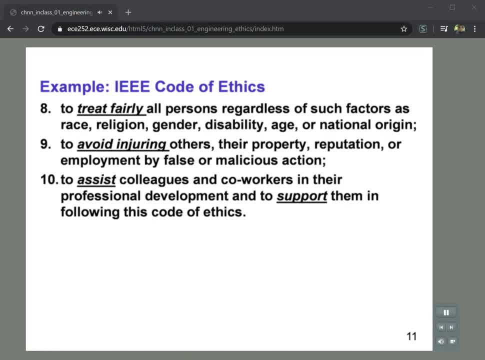 The eighth clause Is really a non-discrimination clause That we should treat fairly all persons Regardless of their race, religion, gender, disability, age Or national origin. This is a standard If you go to work for a big company like IBM. 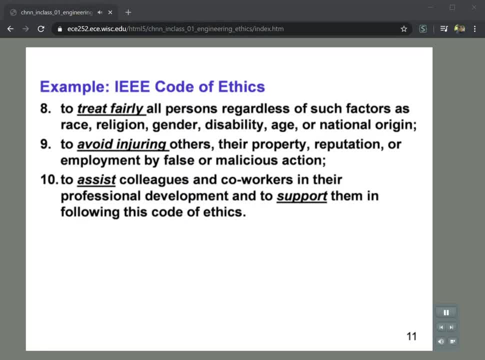 Which is where I worked for a number of years Before I came here. This is something that is very important And was drilled into me Over and over again. This is a firing offense If, in your professional work, You're found to discriminate. 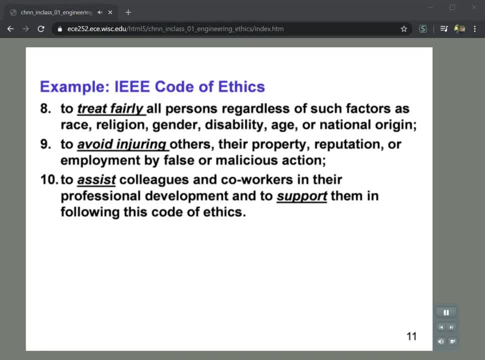 Against anyone On any of these bases. You're probably going to lose your job, And you should. You should engage in Number nine. here is really again Coming back to honesty, But more on the malicious front. So we should never do things. 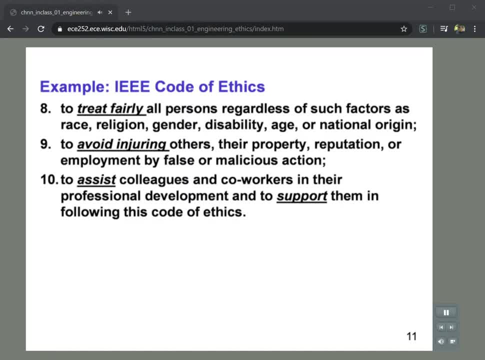 That will injure others, Their property, Their reputation Or their employment By false or malicious action. So this again would be misrepresenting Others and their actions In a context where That misrepresentation will again Affect any of these things. 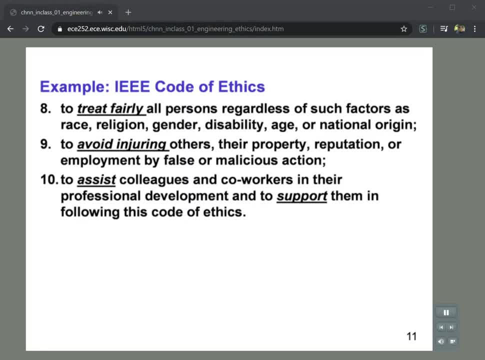 Pretty straight forward. basically Do no harm. And the final clause here is, Again, to be collegial, We should be willing to assist Colleagues and coworkers In their professional development. So if I happen to have developed an expertise In a particular subject area, 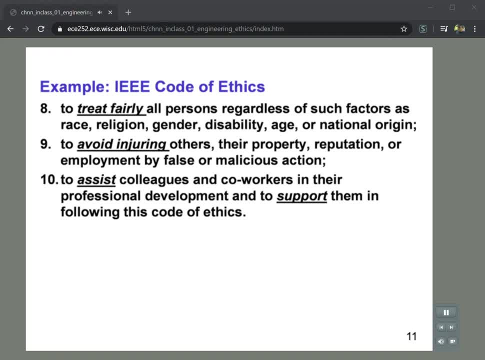 I should be willing to share that expertise With my professional colleagues So that they might better themselves as well. And finally, We should apply this in the context of Following this code of ethics as well. So if we see that someone is, 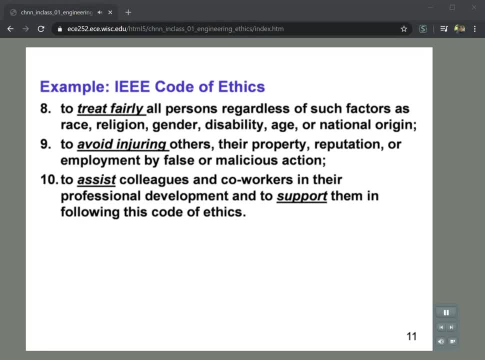 Doing something In response to This code of ethics, We really should be willing to stand behind them. So the common example of this Would be if someone In our workplace Discovers something that Isn't quite right, Isn't quite kosher. 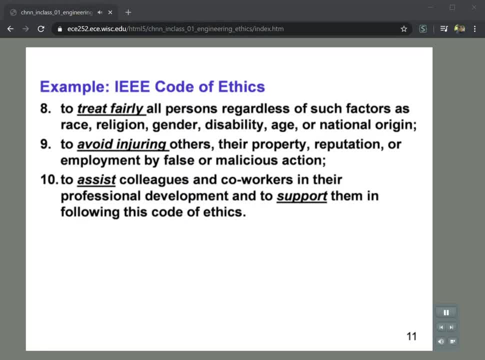 And decides to be what's called a whistleblower. They decide to identify this publicly And sort of Make a federal case out of it. We should be willing to support them In that task. We should be willing to stand up for them. 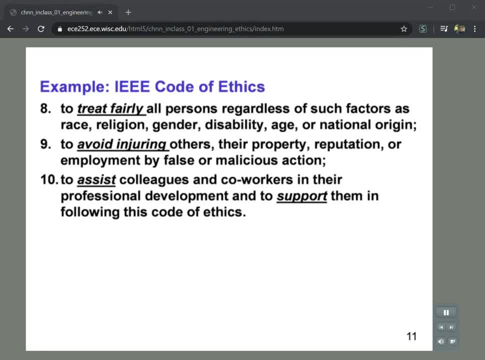 And say they're doing the right thing, And put our own- Basically put our own- careers on the line as well In support of others who are behaving In an ethical manner. Okay, so that's the IEEE code of ethics. Again, it's kind of a mish mash. 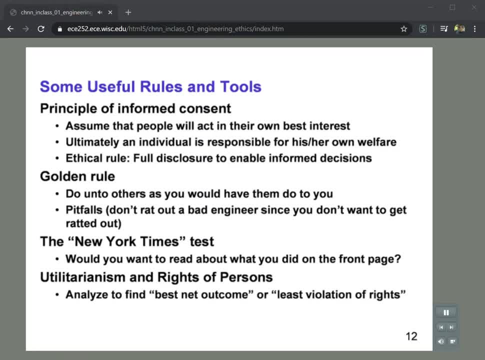 Of suggestions And principles and so on, But it gives you something to chew on, Something to think about The code of ethics That my particular professional society has adopted, Some other things that might be useful, Some of the rules and tools. 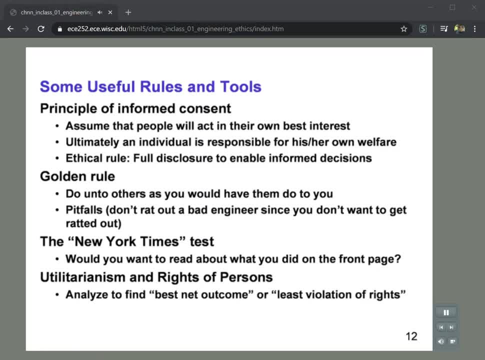 That might be useful Are listed on this slide. I think a really important one Is on the top here. It's the principle of informed consent, And this basically derives from the argument That you can assume that people who are adults, So if you're dealing with adults, 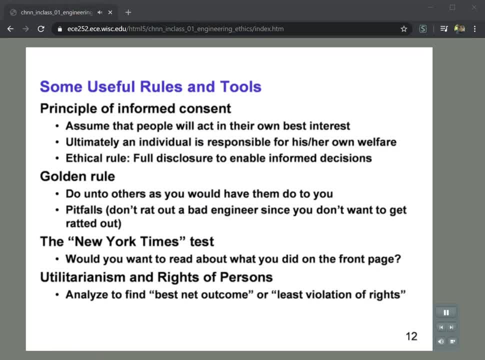 If you're dealing with children, That's a whole other thing. But assuming that you're dealing with adults, They'll act in their own best interest. And they'll act in their own best interest, Of course, If they have full disclosure. 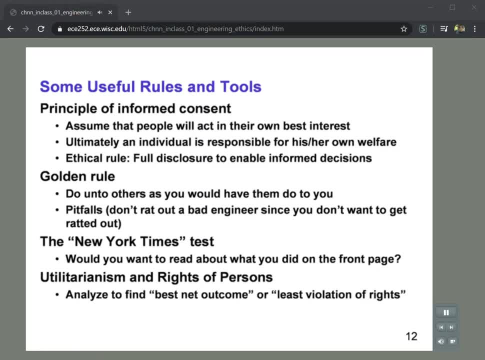 So if they have all of the relevant information at hand, We sometimes just have to assume That people make their own decisions And ultimately they're responsible For their own welfare With respect to that particular decision. But the thing that we can really do, 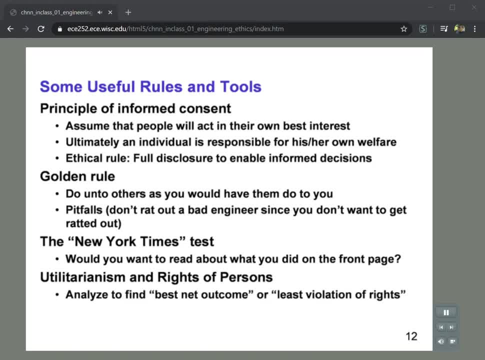 That will mess that up Is to withhold information, And so in a situation where we're going to defer And let someone else make the decision on their own, We really should practice full disclosure So that they can make an informed decision. So we don't withhold. 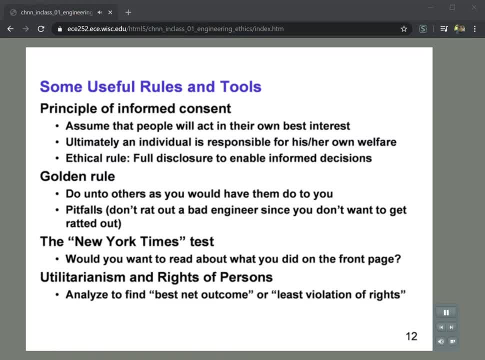 Key pieces of information To steer their decisions in a particular direction. Instead, we give them all the information And say: look, it's up to you. You make your own decision now. So that's, I think, a good principle To remember in all contexts. 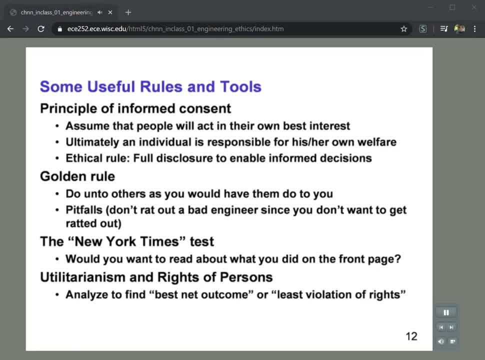 Another one is possibly the golden rule. Just think about it. Think about your actions In the context of doing to others As you would have them do to you If you wouldn't want to have that same thing done to you. Of course, this doesn't always work. 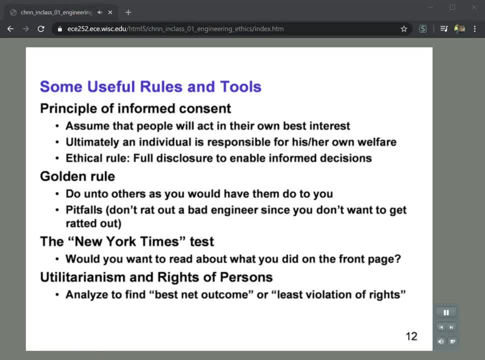 An obvious pitfall would be: You discover that your co-worker Is doing a poor job On a particular project, But you decide, oh well, I'm not going to write them out, I'm not going to make sure this bad design gets fixed. 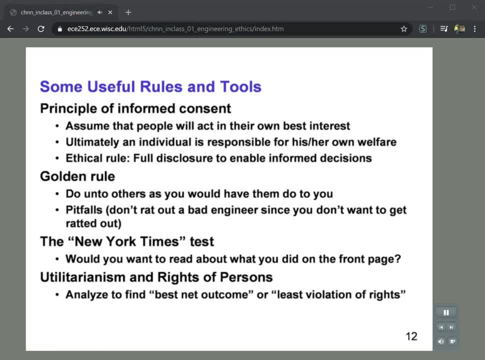 Because I wouldn't want them to do that to me. Well, that's clearly not the ethical outcome, Particularly if the bad work Being done by that co-worker Actually has serious implications On the safety Of the individual, Profitability or any other attribute. 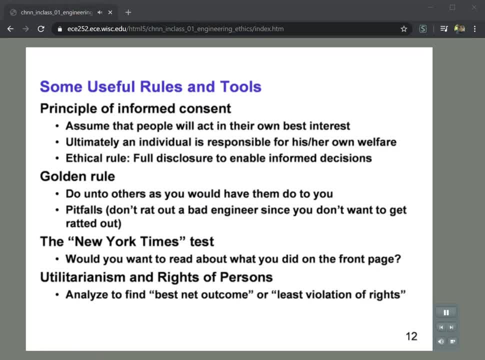 Of the work that that person is doing. Another thing to think about Is what's called the New York Times test: If you're engaging in activities And doing work that You think might end up On the cover of the New York Times. 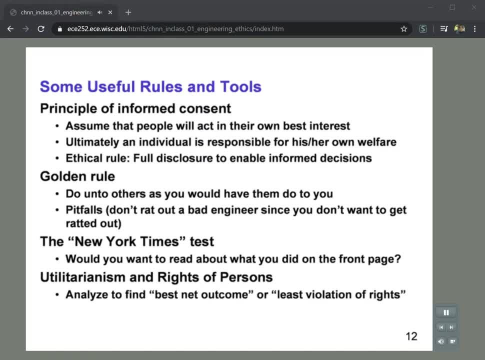 If it comes out into the open. Maybe you should be thinking A little bit more carefully About whether that's something you want to engage in or not. Is the work that you're doing Something that you would want to read about In the New York Times? 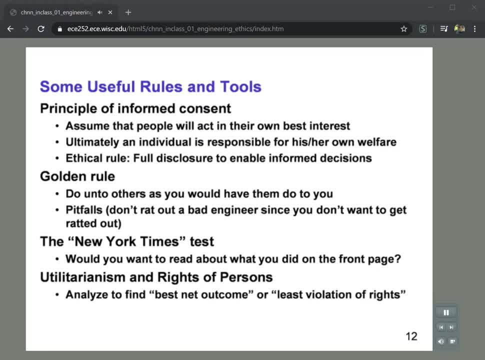 Next week, And not on the front page in a good sense, In a lavatory sense, But in a scandalous sense, And if the work that you're doing falls into that category Or the decisions that you're making Fall into that category, 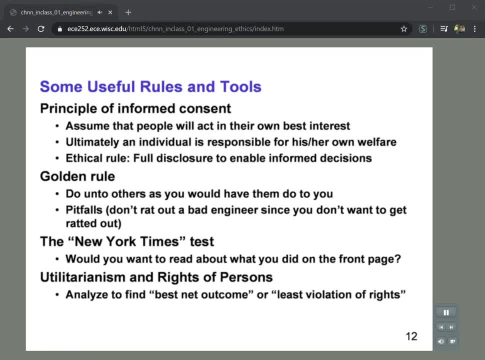 Then you should proceed very carefully. And finally, We'll talk about this analysis process That we can use as a tool, Again, to help identify And perhaps trade off And find the best net outcome Instead of conflicting ethical principles That we're dealing with. 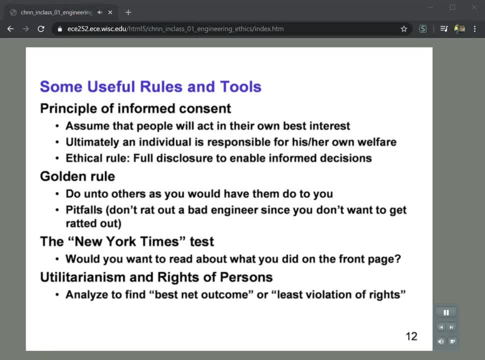 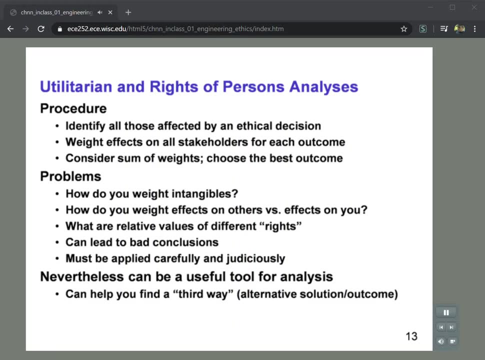 That will lead to the best net outcome Or will lead to the least violation Of the rights of persons As a result of the action That we undertake. So let's talk about this utilitarian analysis, Or it's also sometimes called. 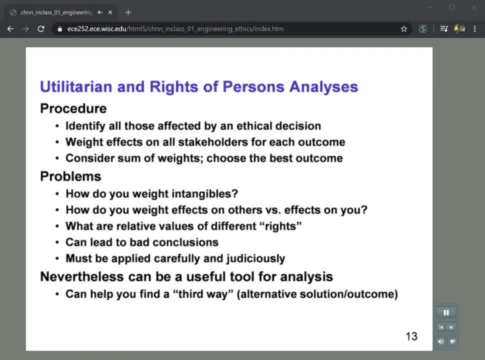 A rights of persons analysis. These two are really very similar, Except one is focused on A rights based analysis. If you're going to do something, It's going to affect someone's right to such and such, But it could also affect some other right. 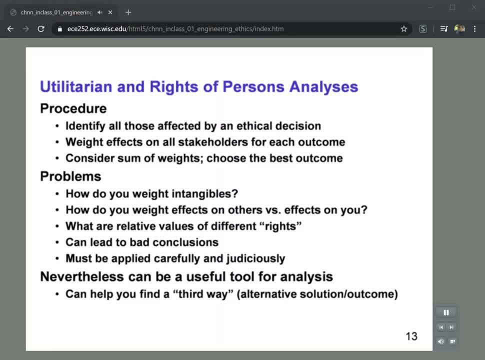 Of some other person to such and such, And so you have to trade off these rights against each other. Or, from the utilitarian perspective, You can sort of place weights And effects, Assign weights and effects to all outcomes In your decision process. 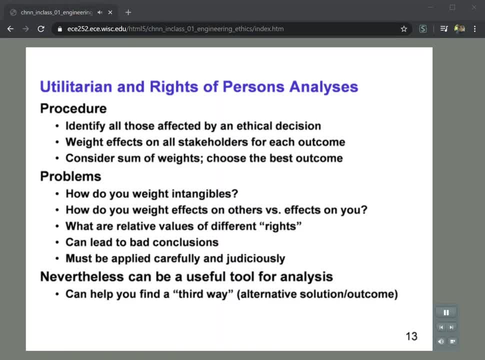 And then consider the sum of all the weights And choose the one with the best outcome. So the procedure really is: You identify all those individuals or entities That are going to be affected By the actual decision that you're trying to make. 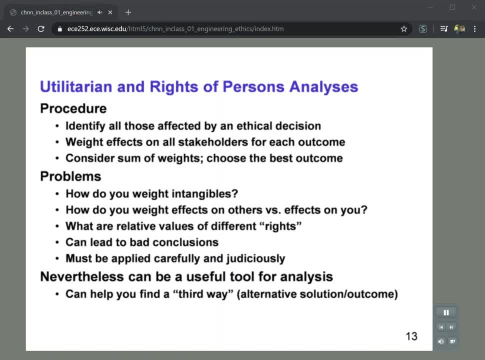 And you have to then weight the effects On all the stakeholders For each possible outcome That you might reach And then consider some of these weights And use that as a way of guiding you Towards choosing the best outcome. Now, unfortunately, 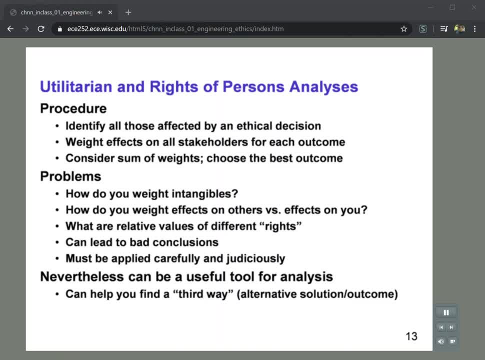 This is not an algorithm. It's not going to give you the right answer. It may even lead you down the wrong path. Potentially, It's really just another tool That allows you to critically analyze And introspectively think about. 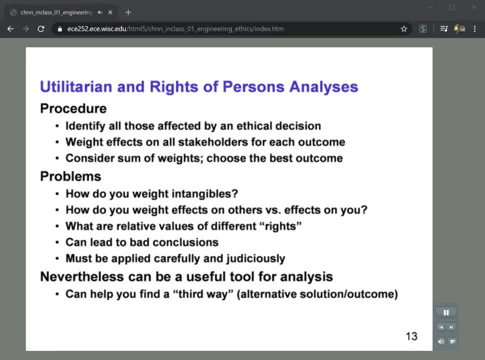 The situation that you're facing Rather than simply rushing To a gut level decision. And some of the problems that arise here are: If you have intangible benefits Or intangible Negative effects, How do you weight those? How do you weight the effects on one person? 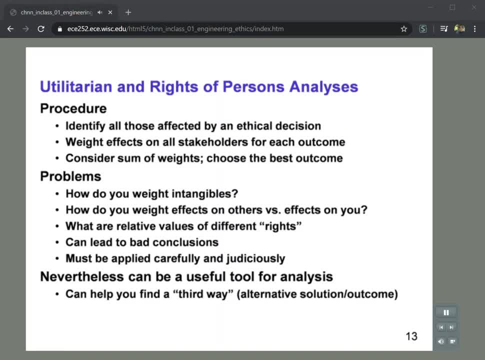 Versus another person. It's hard to say how important a particular effect might be On different individuals. And what about these rights of persons? How do you place relative values On them? So you have to be very careful about staring at a number. 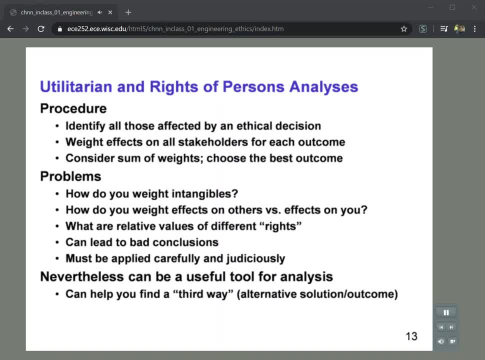 And saying: oh well, look at this number. This number is greater than that number. Therefore, this must be the right answer. No, We're really in the realm of unquantifiable Quantities here that Are very difficult to To analyze. 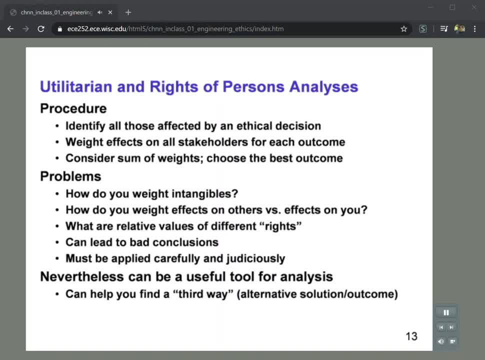 To that extent, To that quantitative extent. So we have to be careful about applying This kind of analysis To ethical situations Really carefully and judiciously, Just as a tool for analysis That might help you find, Potentially, an alternative solution or outcome. 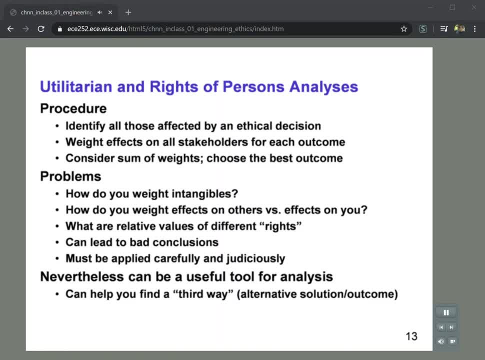 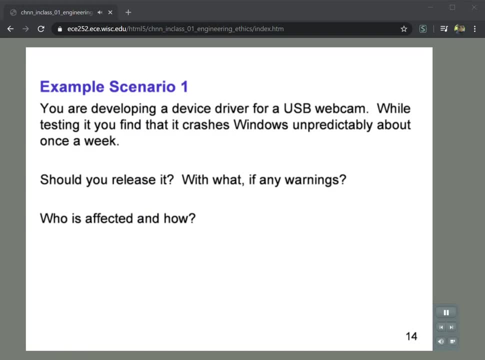 That is maybe one that you hadn't thought of Up front. That might be some sort of compromise That ends up Minimizing the negatives, Maximizing the positives Of that situation. Let's go through a couple of Example scenarios. 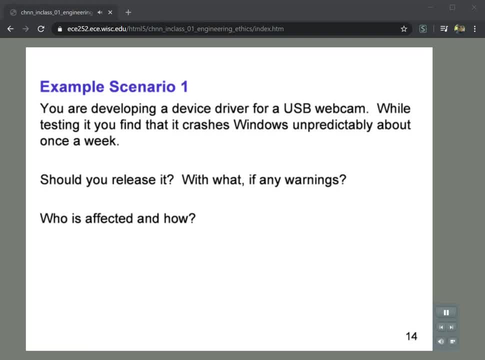 Just to help make all of this mumbo jumbo A little bit more concrete and clear. So this is a pretty, Pretty straightforward one That's pretty relevant to the topical material We've been covering in this course. So let's say you're working for a company. 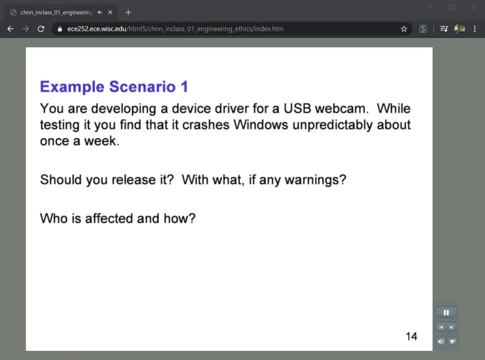 That's developed a new USB device That plugs into people's computers- It's a webcam in this case- And you're responsible for writing a device driver, A piece of the operating system That actually interfaces at a low level To that IO device. 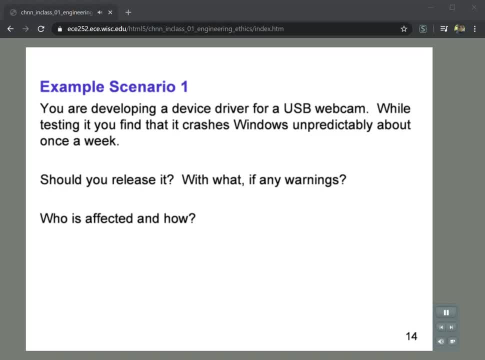 You've been working on it for a while And while testing it It does a crash, unpredictably, About once a week, So it'll typically run for about a week Before it causes any problems. Now you're under a lot of pressure. 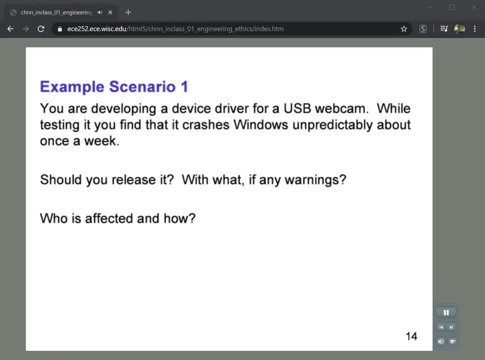 From your manager. You've got to get this device driver out the door, Because it's the only revenue product That your company has, And if you don't start shipping it soon, Your company might go out of business. So what should you do? 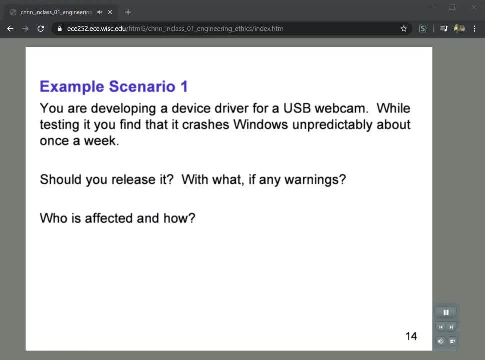 Should you go ahead and release this device With this device driver? That doesn't quite work 100% of the time. What tools should you put on it, And who is affected, and how, By the decisions that you make in this process? 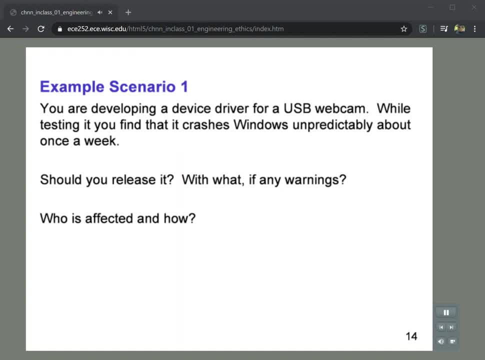 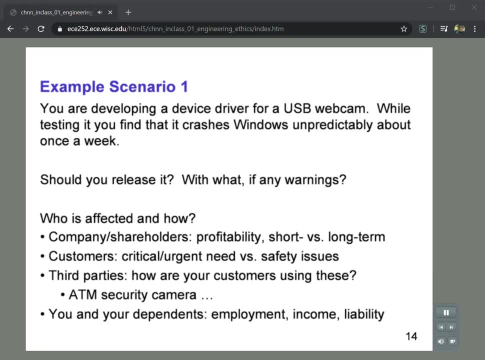 How do you even begin to think about this? So let's step back And think about our analysis approach And say, okay. First of all, let's identify the stakeholders In this situation, And I can think of at least four categories. So first of all, the company. 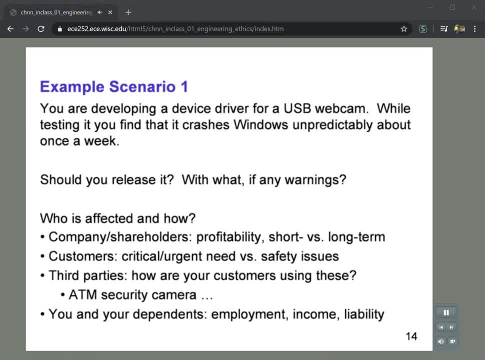 Which may have shareholders Who've invested in it. They're obviously concerned about profitability In the short term, But there's also a long term issue here. If you ship a defective product, That might kill the long term prospects of your company. 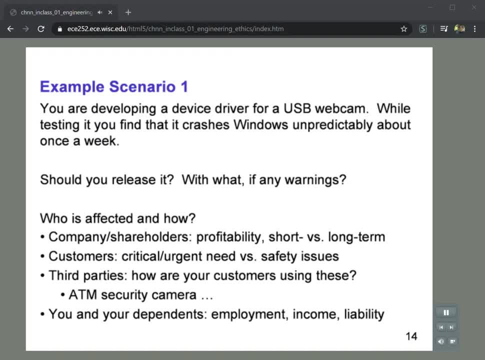 If enough customers are Affected negatively by this, Your company may end up folding. If the product is too shoddy, There's also the customers. There may be some customers out there That have a critical or urgent need For this particular device. 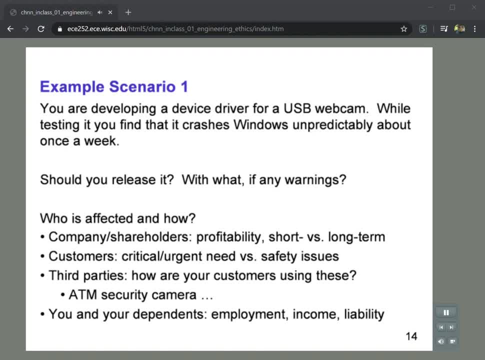 So Maybe it's actually important for them That you get this out. They've been waiting for this And they really need it, And if they don't get it soon, Then whatever they're trying to sell, Maybe it's a service that they're selling. 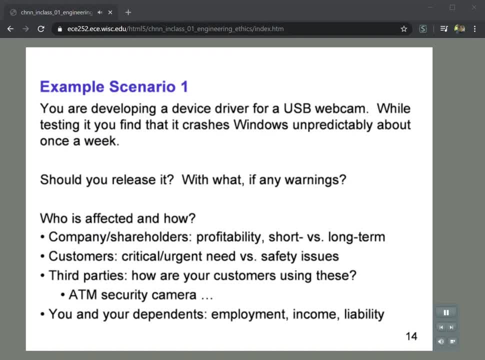 Or maybe it's another product That integrates your product into it. They're going to be delayed And they're going to be in trouble, So maybe there's an issue there. On the other hand, The customers, who are actually end users of this device- 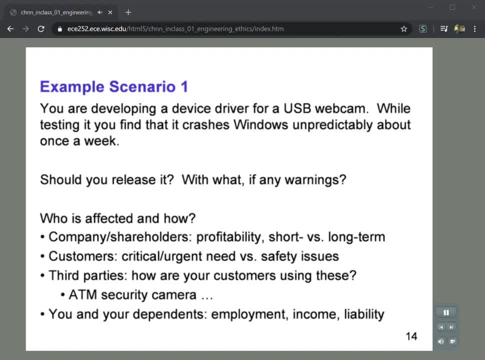 Might face safety issues If they rely on this particular computer That they connect this webcam to To perform some safety critical task And crash their computer once a week. Potentially, very bad things could happen, So you have to take those into consideration as well. 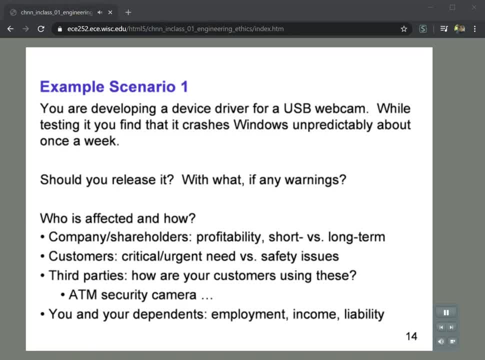 There are also third parties. Maybe your customers are using these In applications That you haven't really potentially envisioned. What if somebody is actually Going to incorporate this Into their ATM as a security camera? So their ATM runs Windows. The ATM needs to have a security camera. 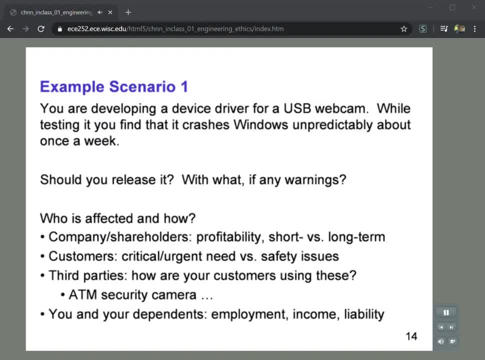 To film, Create a record of everybody who uses the ATM. They're going to use your USB webcam In this product. Now the ATM is going to crash Once a week As a result of your USB webcam's device driver Being flaky. 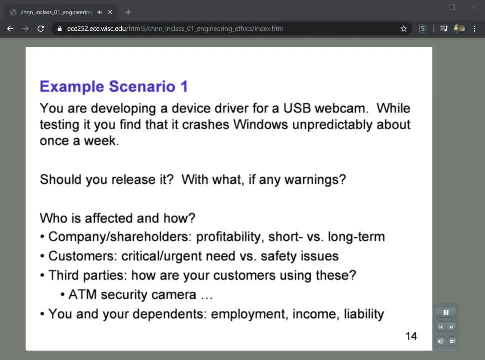 What does that mean? What are the implications of that? Well, if the ATM crashes in a way That no one can use it anymore And no one can get any more cash out of it, Maybe that's okay. That's mostly an inconvenience to anybody. 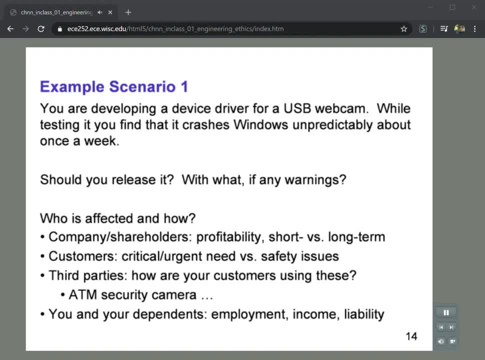 That might want to use that ATM. However, it could potentially crash in a way That no one can afford it, And so there's a financial loss now For the bank that's using that ATM, And so on. So there might be all kinds of scenarios. 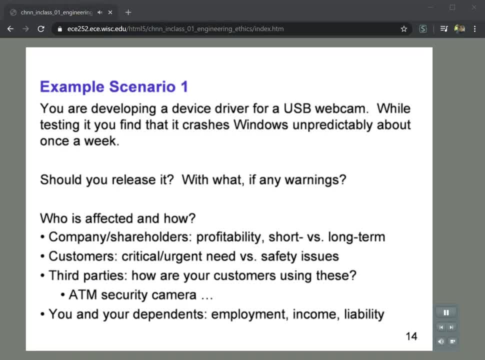 That might arise, Based on the different kinds of usages That customers will actually put your device to. So you have to be again Aware of these things, You have to think about them Before you can really make an informed decision About how to proceed. 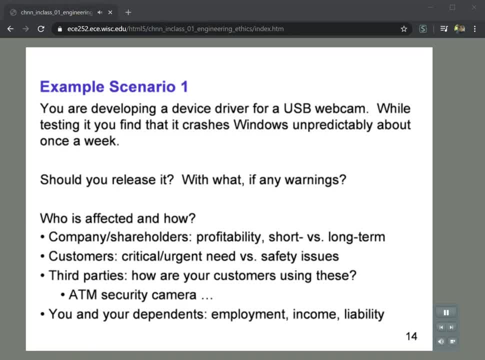 Finally, of course, You and your dependents are always involved. If you actually ship a defective product, There could even be legal liability issues That might come back to Hurt you and your family Later on down the road. So you can imagine that a fairly simple scenario here. 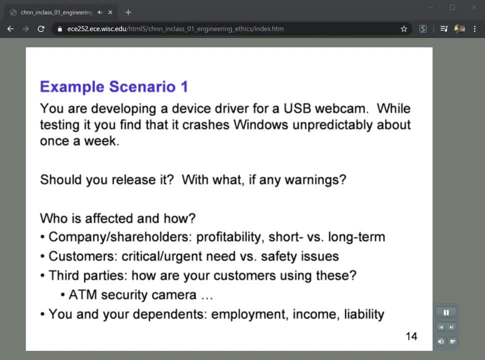 That seems pretty straight forward. Actually, from an ethical perspective, Can get pretty complicated, Even just from the perspective of trying to identify Who are the individuals that are affected Or the entities that are affected. How are they affected? What, again, are the ethical principles? 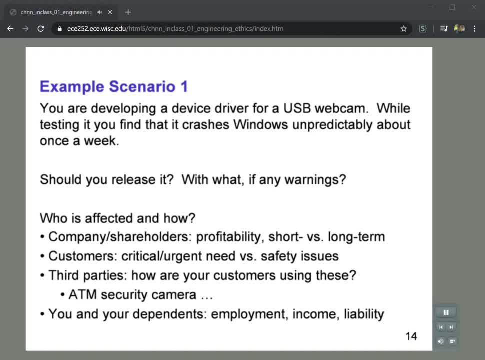 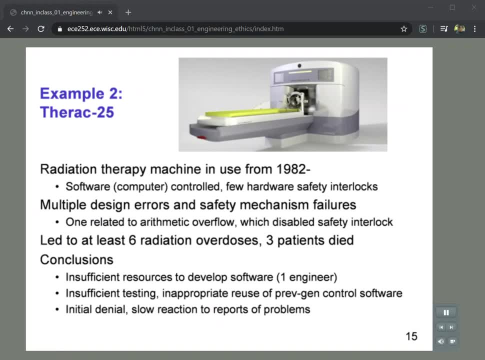 That we're going to be running into here, That we have to, That we have to trade off against each other And figure out what is the right thing to do. Next. we have a real example. This is kind of a sad story. 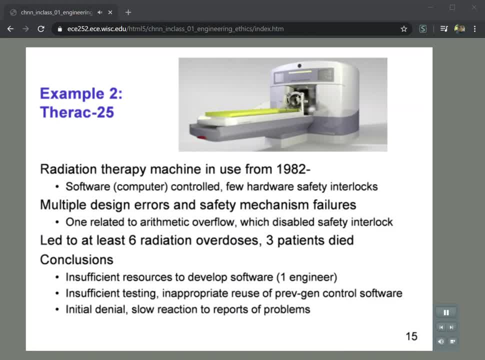 The Therac-25. Was a radiation therapy machine That was in use from 1982 on. It was a machine that was developed in France, So this was obviously used for cancer treatment, To provide radiation therapy To try to kill cancer cells. 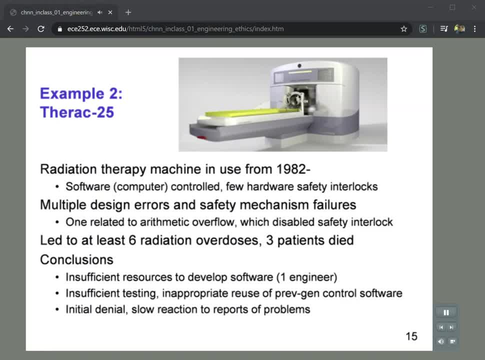 It was the first machine That was developed in the United States. It was the first machine, The first device of its kind That was software computer controlled. It had very few safety interlocks Directly built into the hardware. It was assumed that all of these safety interlocks 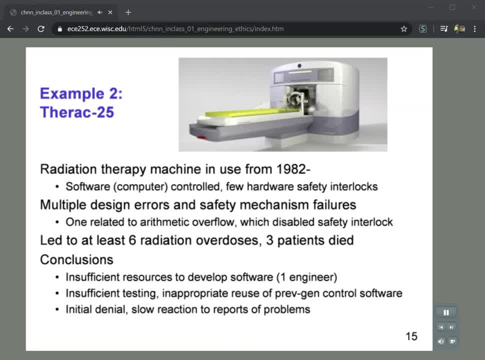 Would be in the software itself. Now it turned out That the software That was written for this device Had many design errors in it And many safety mechanism failures in it. One of them, coincidentally, Was related to arithmetic overflow, Which we studied earlier in this course. 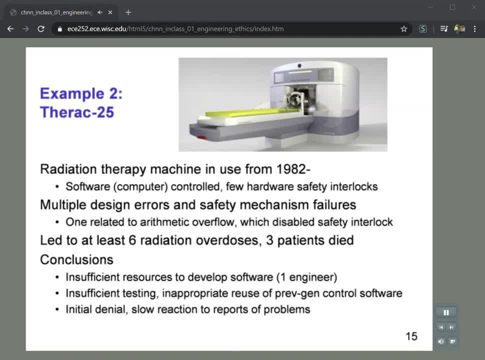 And that overflow condition Would allow dangerous levels Of radiation dosages to be applied To patients. Ultimately, this led to at least six radiation overdoses. Three patients died As a result of these failures And the conclusions That came out of the study. 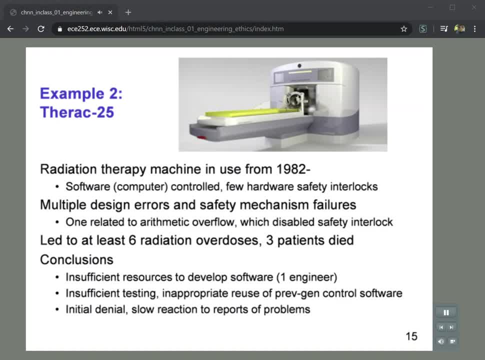 That was done to understand What went wrong, Where that the company had really Applied insufficient resources To developing the software for this machine. They really just had one programmer And one engineer working on it And they had insufficient testing Of that software. 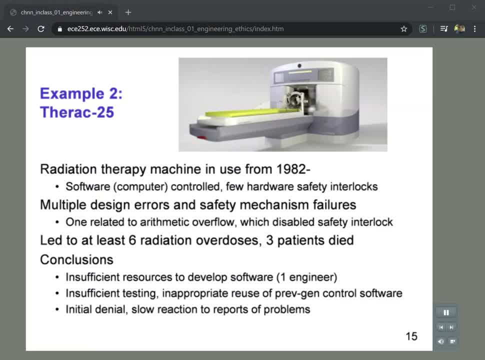 There was inappropriate reuse Of previous generation control software. So there was a previous generation machine That actually had hardware safety interlocks in it. So the control software Didn't enforce those safety interlocks, They just simply used Pieces of that old control software. 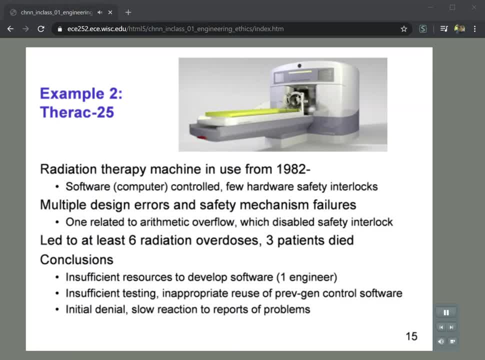 In the new generation hardware. The new generation hardware Didn't have any safety mechanisms built into it, And so these disastrous, Disastrous overdoses of radiation Became possible. Also, there were problems on the management front. Initially, the company denied any problems. 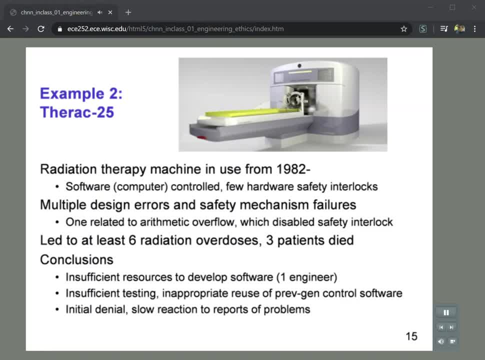 They had reacted very slowly To reports of problems, And so many more patients Were exposed to these problems Before they were eventually fixed. So again, This is a concrete example Of somebody writing software And making some very serious mistakes And not being very thoughtful. 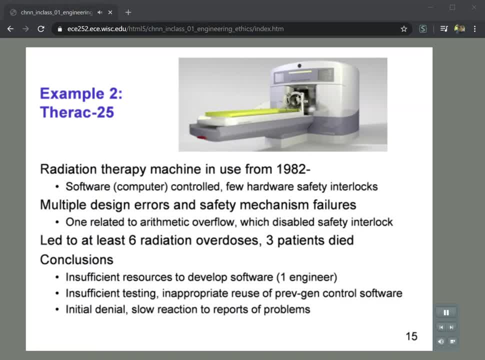 Not being very thorough, Not being very careful Of the result Of this carelessness. So this should be a reminder here Of the potential for severe consequences If we don't, If we don't conduct ourselves In our professional lives. 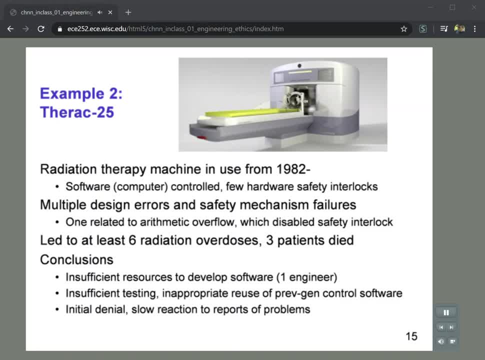 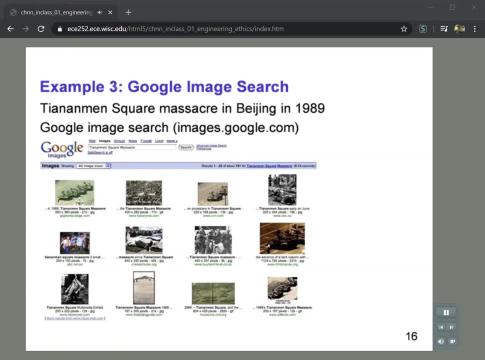 In a way that, In a careful, thoughtful, ethical way That we should, That we should conduct ourselves. This final example here Has to do with something that Came up just a few years ago, So hopefully You're familiar with the Tiananmen Square Massacre. 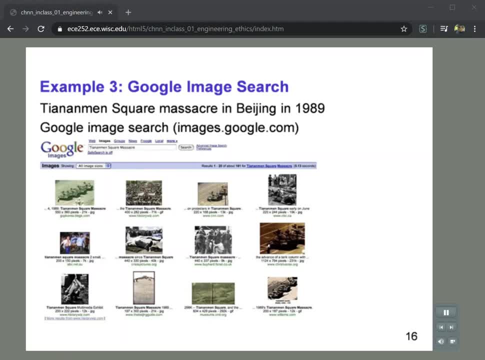 Which happened in Beijing In China in 1987. This was a protest that happened In this public square, Where the Chinese government Sent in the Red Army Tanks and everything To basically Quench this protest And a bunch of people died. 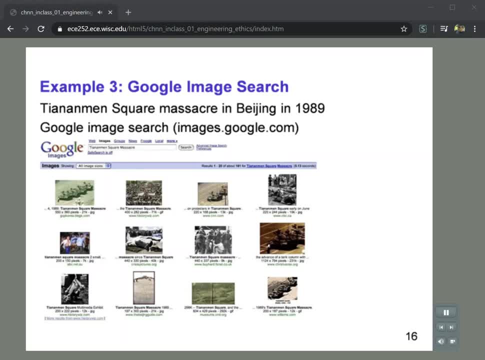 As a result, And as you can see in some of the pictures On this webpage, If you do a Google image search For Tiananmen Square Massacre, These are the kinds of pictures That turn up, So you see the tanks. 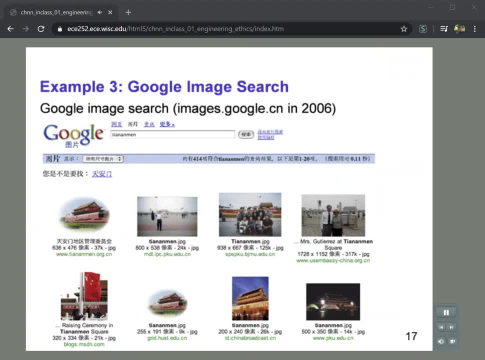 You see people being beaten down And so on. Now the interesting thing is That if you actually do the same search, If you search for Tiananmen Square On the Chinese version Of the Google image search site, Imagesgooglecn, This is the site that's accessible within China. 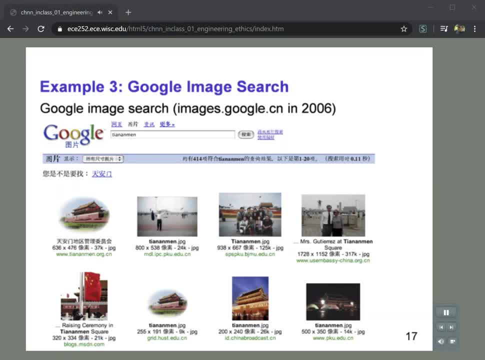 Or at the time back in 2006.. Was accessible in China. Instead of seeing pictures Of protesters being beaten down And tanks and so on, And soldiers, This is what you get. You basically get a collection of people's tourist photos. 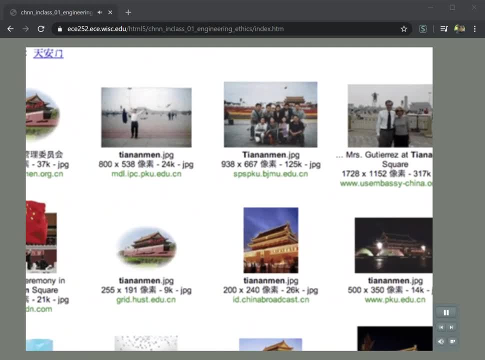 From Tiananmen Square. So if we zoom in on that You can see those a little bit more closely again. So these are all very peaceful And happy And wonderful pictures. No clue that anything bad had ever happened In Tiananmen Square. 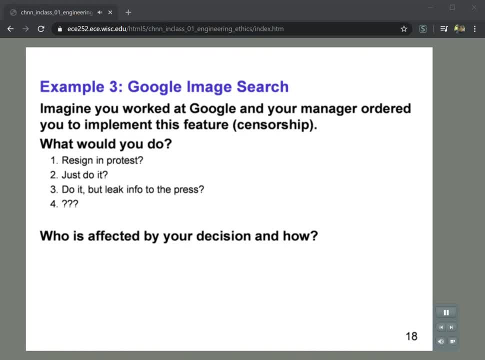 So how can this be? The same company Implements an image search And the images that come up Are so drastically different Depending on whether you're doing the search within China Or whether you're doing the search within the US. Well, the only way. 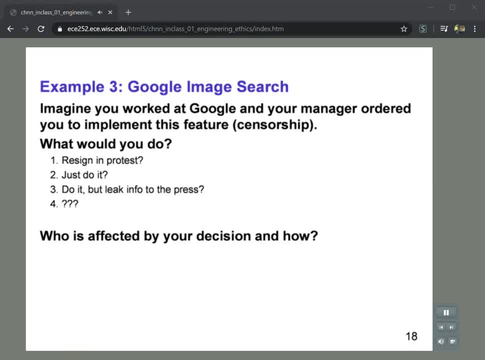 That this could have happened Is by design, So somebody at Google, In Google's management chain, Made the decision That this was the right thing to do Was to censor these images, Which are invisible To residents of China Who are doing Google searches for Tiananmen Square. 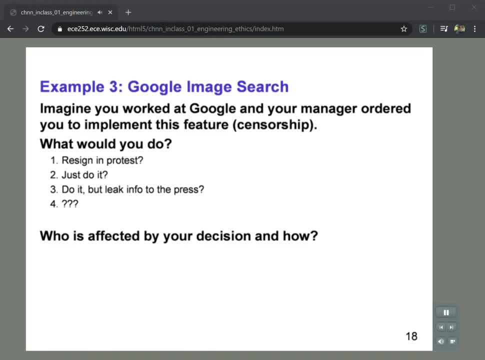 They basically want to erase this event From their memory. They don't want people to know about it. Obviously, Google had to collaborate and agree With the Chinese government In terms of implementing this censorship. Now imagine That you Sitting in your cubicle at Google. 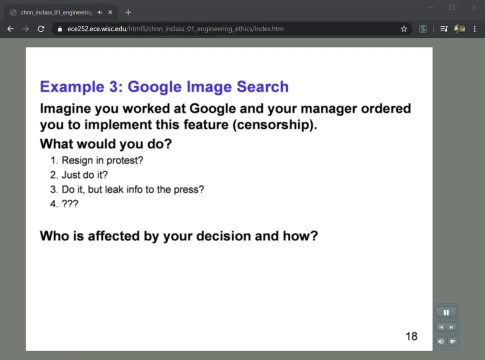 You just got this great job. You're happy to be working at this very successful startup company And your manager walks up to you and says: I'm going to enable image search in China. And, by the way, The government has told us. 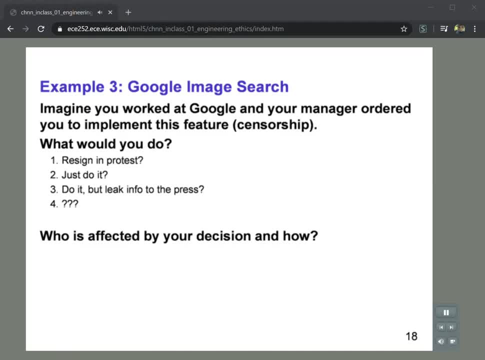 That we can't make these particular images available. So you're going to be now writing some code To make sure that anybody That searches for Tiananmen Square Within China Is actually going to get a different set of results From people who search for it outside of China. 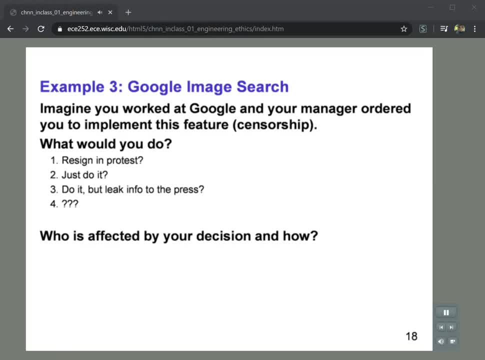 Ethical situation. What would you do? Are you comfortable with this? Are you comfortable with this censorship? Would you go ahead and do that? Would you resign in protest? You'd be so upset that you'd quit your job. Would you go ahead and do it? 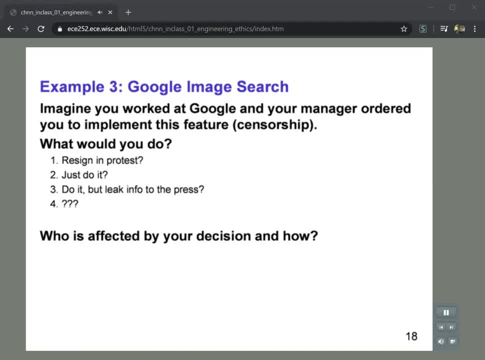 But you would leak the information to the press So that there would be an uproar, As there was when this was leaked, Or would you follow some alternative path? So let's think about this: If you make this decision, Who's going to be affected by your decision? 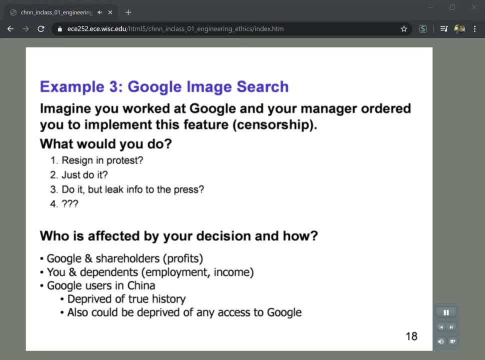 And how are they going to be affected by it? Well, obviously Google itself will be affected And shareholders and investors in Google will be affected, Because obviously Google wants to be in China Because there's profits to be made. It's a huge market. 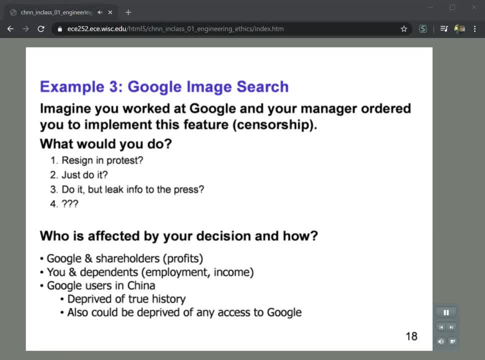 And they don't want to be shut out of that market. You obviously will be affected as well- You and your dependents- Because if you refuse to do this, You'll probably get fired, You'll lose your employment, You'll lose your income. 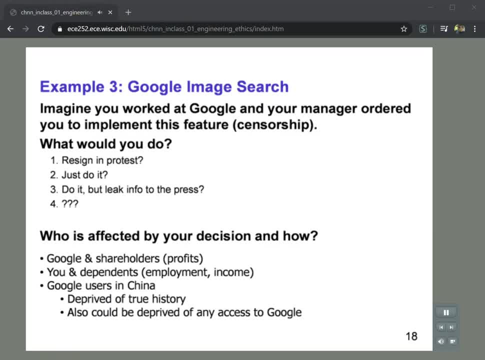 But on the other hand, There's also Google users in China. If you implement this censorship feature, They're going to be deprived of the true history Of the events of Tiananmen Square And they'll be helping A totalitarian government. 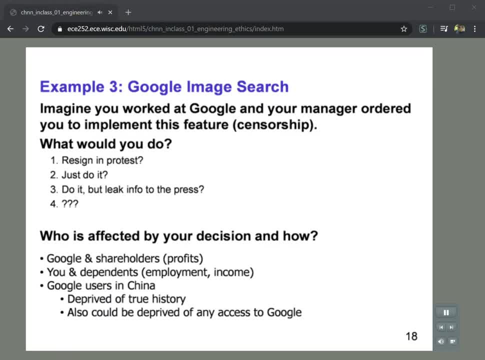 Repress this piece of their history. On the flip side, If you decide to protest And decide that you're not going to follow through On the censorship task, Probably what will happen is The Chinese government will say to Google: Well, we're not going to allow you any access to our market. then 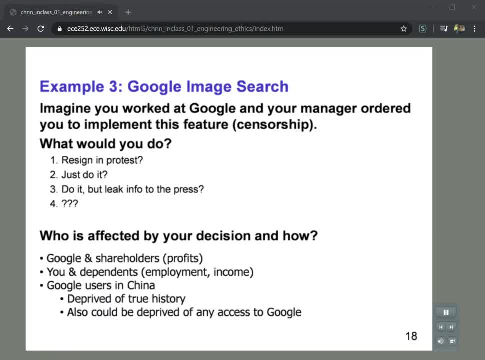 And Any internet user then In China Will be deprived of any access to Google, And that actually has negative consequences as well. In fact, I think this, I believe this- was the main justification That Google used at the time To actually allow this kind of censorship to occur. 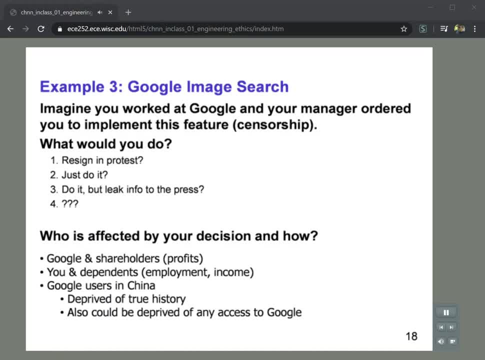 Was that the net benefit Of providing Chinese users With access to Google Outweighed the net negative Of censoring a small part Of the history of China In those search results. So again It gets pretty complicated. There's positives and there's negatives. 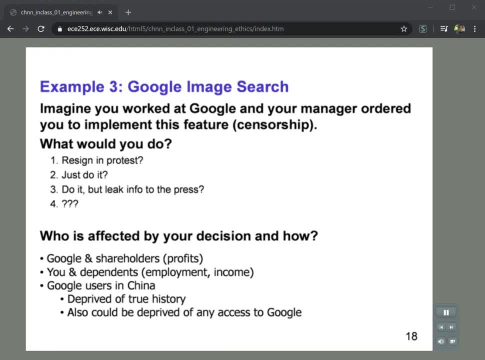 But it's the right thing to do. What would you do? I can't tell you the right answer. If I had been presented with this situation, I honestly can't tell you what I would have done. It's never that simple. It's never that black and white.